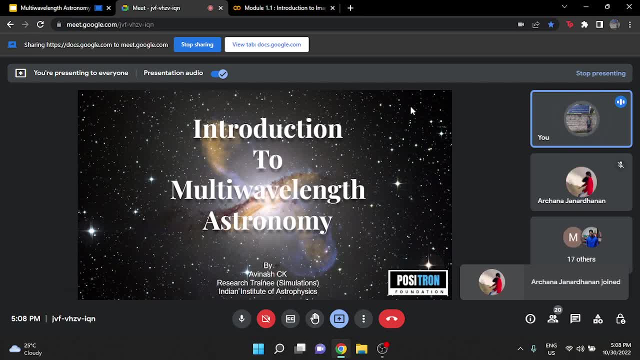 one thing is learning to code, and to do coding is a very different thing. If you know the basics of a programming language, everything comes down to the programming logic which comes out of practice. So if you are learning a new library, for example, say AstroPy or Fort Utilis, if you 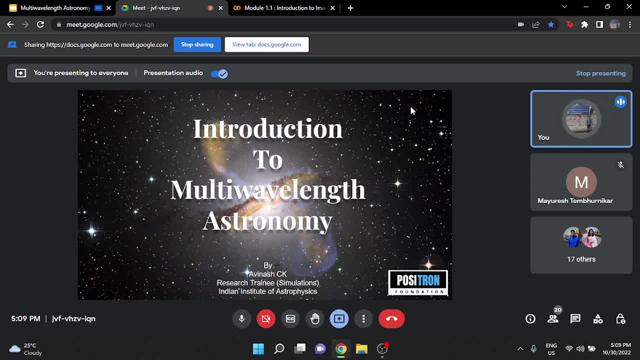 understand the programming logic and you have some idea of how to play with the code, then it's actually very easy to learn any new package. So initially, in the first week, when most of you just opened the notebooks, I think a lot of you got scared because it looked completely random and new. But I'm actually happy to. 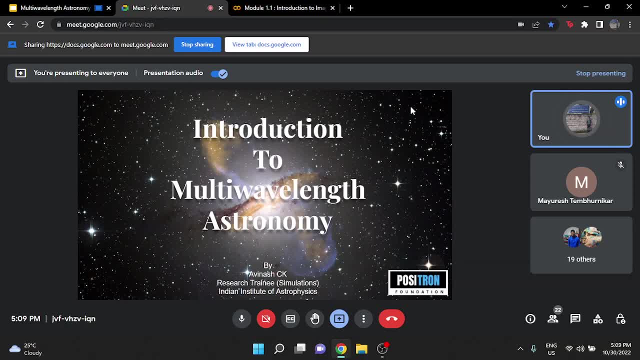 tell you that a lot of you have solved. The number is comparatively much higher than what we had in the first week in the last two sessions. Maybe it's because this time we screened and tried to make sure only the people who are actually interested participate in the course. 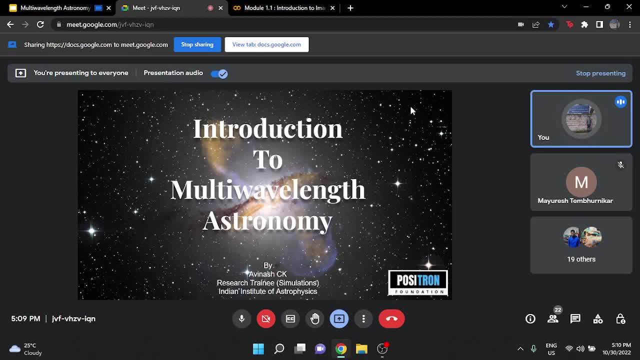 But I think the point is put across to most of you, because we see that many of you played with the code, came up with different multiple solutions and explored and noted down your own observations. But if I think, even though many of you solved it, some of you still haven't got what we 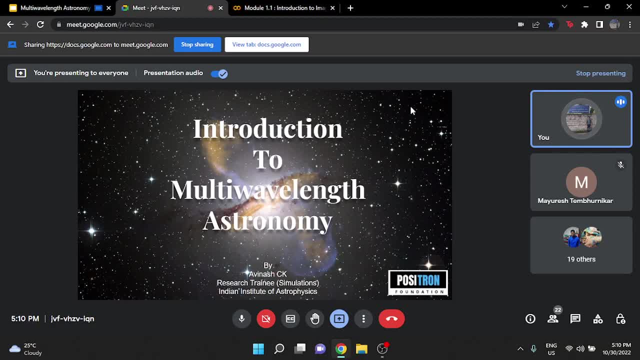 were going for. but you don't have to worry. If you have coding difficulties, we'll help. We are more than ready to help you with that. Many people have benefited from the four of us in the course of last one week. So, coding wise, the one-week length is given so that you have enough time to explore and 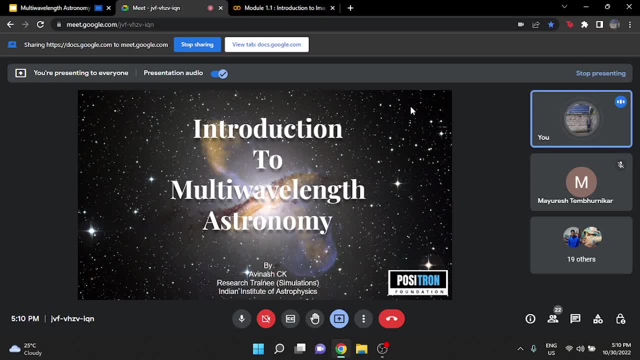 You don't have to worry if you're not getting the solution and you have to make mistakes. And that's the most important learning from this exact alternate approach to learning. And it is based on this one tidbit that I found out from Richard Feynman's book on Surely. You Must Be Kidding, Mr Feynman. 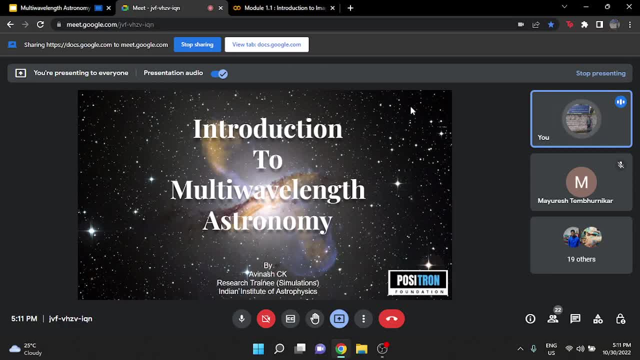 And there he talks about. when he was in college and in school, he used to do this one thing where he hears a word or comes across a topic that he hasn't heard before. He tries to do this one thing where he tries to guess what the topic is or guess what the concept is. 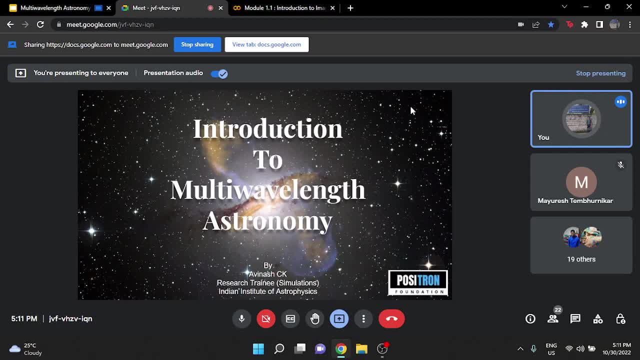 Then, once he has set up his mind, then he goes and reads about it, then finds what it is actually. So what it does psychologically is: you have what it is and you have a list of all the things, But it is not So it sort of embeds in your brain much better. 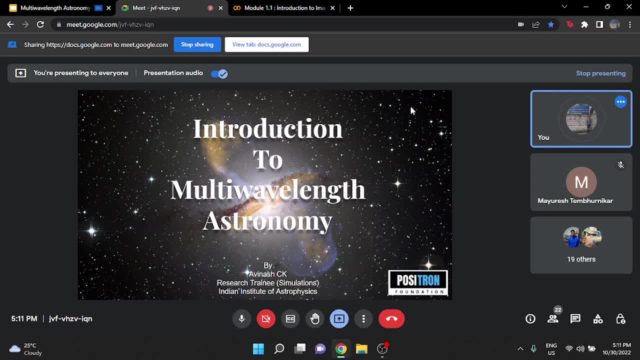 So through this lecture the goal is actually to connect whatever is in the module. We surely will be discussing the coding part, So if you didn't get the puzzle solutions or you're stuck somewhere, we'll go through that also at the end of the lecture. 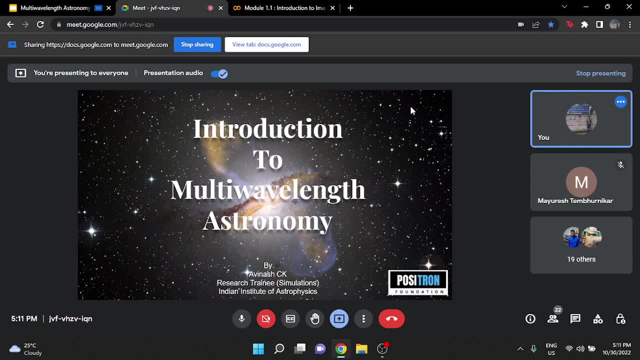 But through this introduction to multivariate astronomy lecture, my aim is to show you why did you do what you did and what. what is the impact On the scientific impact on this study, like what all can be done using the methods that you explored and what has been done using these methods? 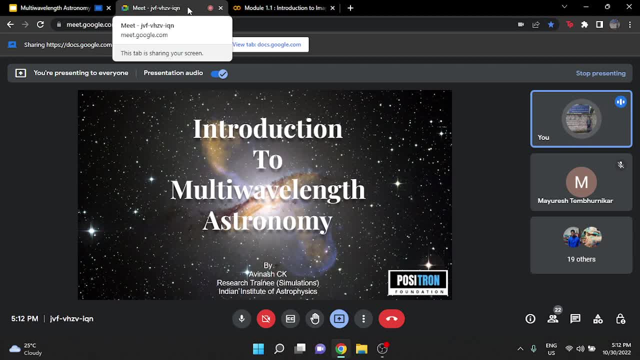 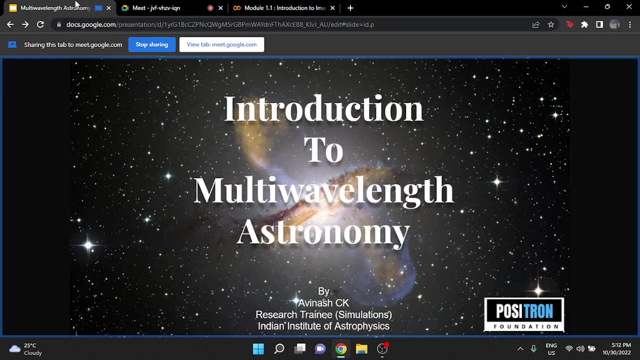 So let me start. So if you are with me, can you drop a yes in the chat, Like if you are OK with me proceeding ahead, OK, great. So I want to tell you that if, at any point, if I'm rushing through or going very fast or you want to, you want to get. 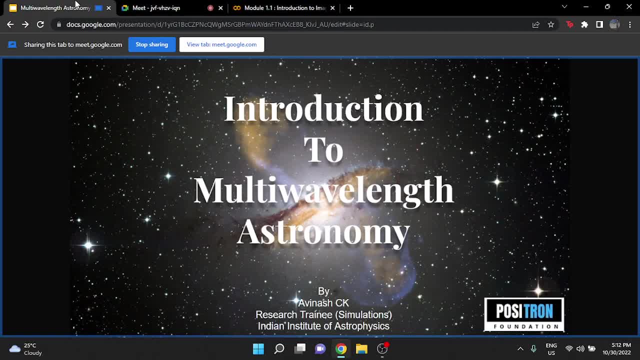 Much a bit more clarity on any topic. you can stop me any time in between. I'm actually trying to record the sessions for the ones who have network issues and the ones who couldn't make it to the class. But in case we can't, you're not able to record or the recording is not proper. 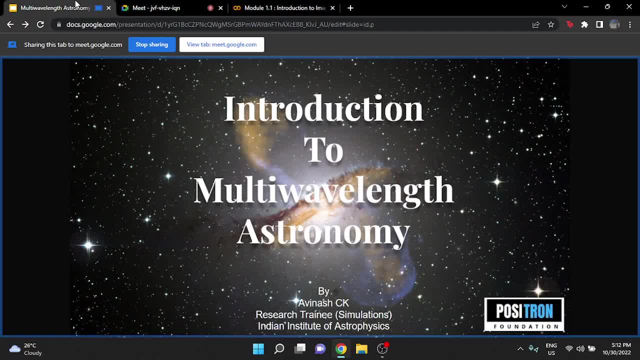 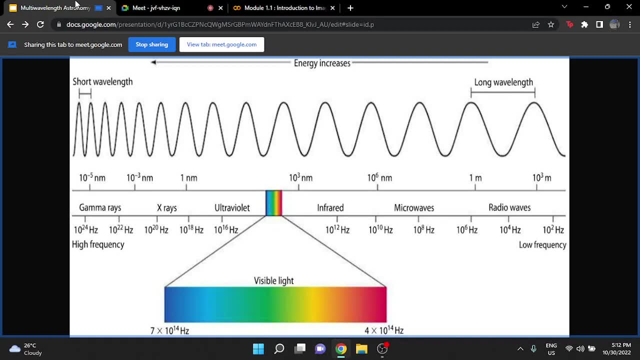 So I suggest that you can stop me any time you have a doubt, So I'll begin. So, as you all must know by now, the primary source of information or data that we have in astronomy is through light. So, as you all must know by now, the primary source of information or data that we have in astronomy is through light. 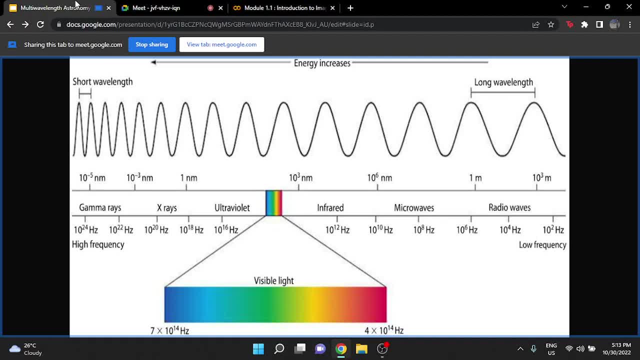 And from our very basics in college education and school, we know that light is part of the electromagnetic spectrum and that light is the electromagnetic, is an electromagnetic wave, And we know that it's other than what we perceive, which we classify as a visible light. 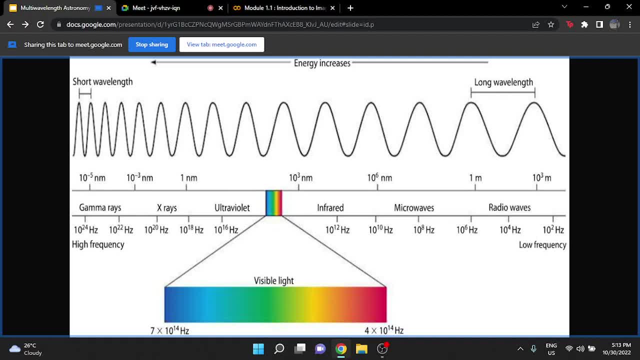 There is an entire other classes, entire class of different bands of spectrum that we studied at different portions in our academic career. So we must have heard about gamma rays, x-rays, ultraviolet infrared microwave. So all of this is part of the electromagnetic spectrum. 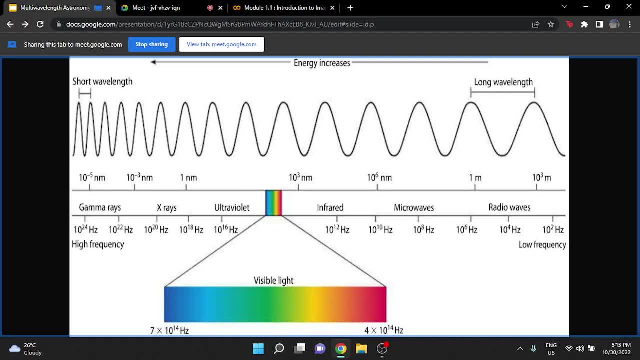 So, but we humans are limited to the visible band, So it's not special Why visible. It's only that we are only able to see this portion of the electromagnetic spectrum, And there's actually a very interesting reason why that is So. I'm not sure how many of you must be knowing. 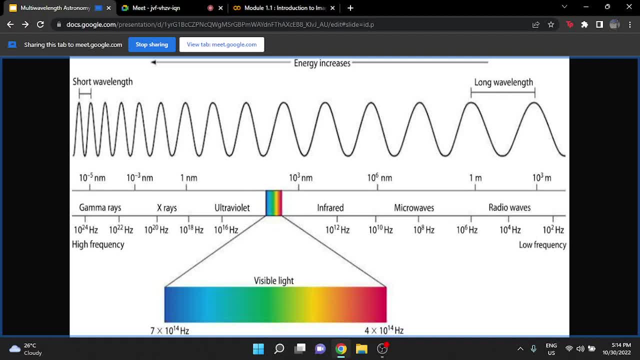 So if you look at the solar spectra, The sun's surface temperature is about 5000 Kelvin And, if you like, check the corresponding blackbody temperature, that which is using the blackbody temperature. if you find the corresponding peak wavelength, it falls in the middle of the what we call as the visible spectrum. 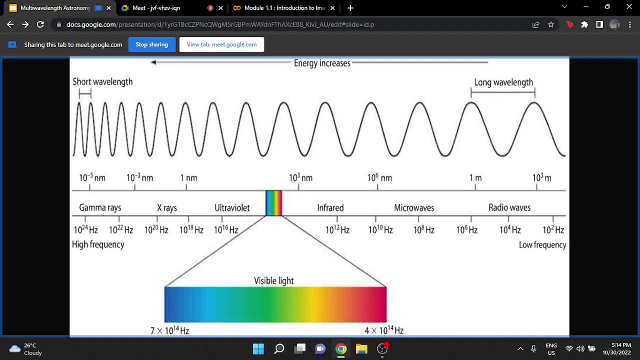 So the reason, sort of why everything on Earth is around visible spectrum is because, actually, of the sun's spectra. It's because sun Peaks at optical spectra, So in order for plants to have maximum power, transfer, it naturally adopted to the wavelength where the sun is emitting, the more 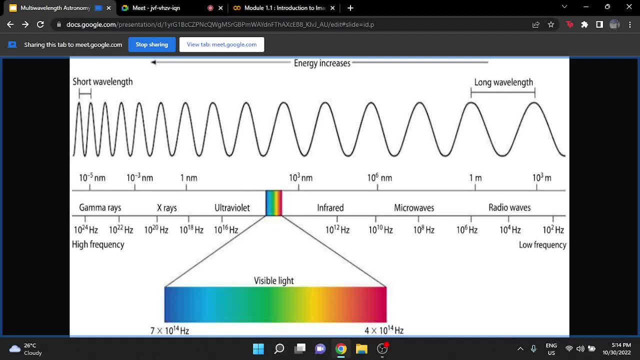 So it's so if you apply that logic. if you were in a solar system where the star peak didn't say ultraviolet, the creatures there would have had sort of pupillary devices. if may, would have been able to See the entire universe in ultraviolet. 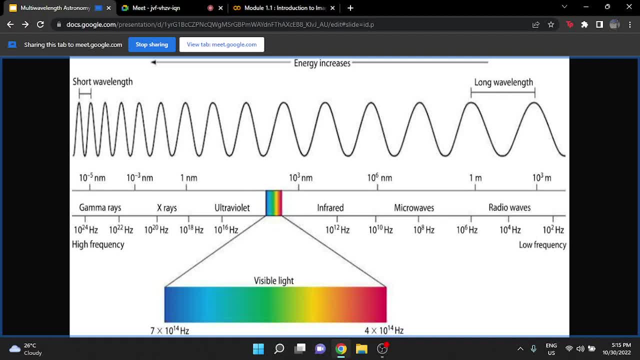 So it's interesting that how much of our surrounding is dependent on how we are like, how what is the surface temperature of the sun and what wavelength it emits. And it's interesting that now we are living in a period where we understand what sort of why, the reason some of our like the things that we see on Earth, why they are the way they are. 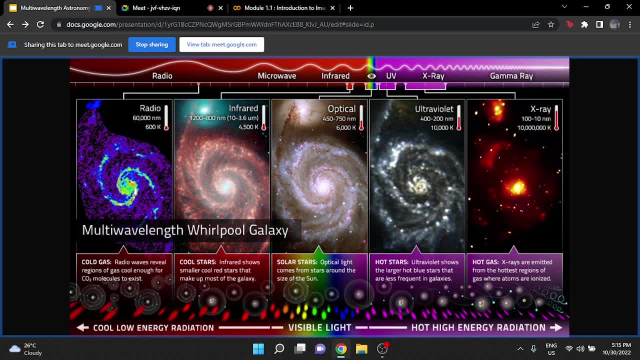 So moving ahead. So, As I said, we are only able to see the universe, like in the surrounding and optical. that doesn't mean there is nothing interesting happening in the other wavelengths. So when we look at the universe we look out from Earth, look into other galaxies and we look at different electromagnetic bands. 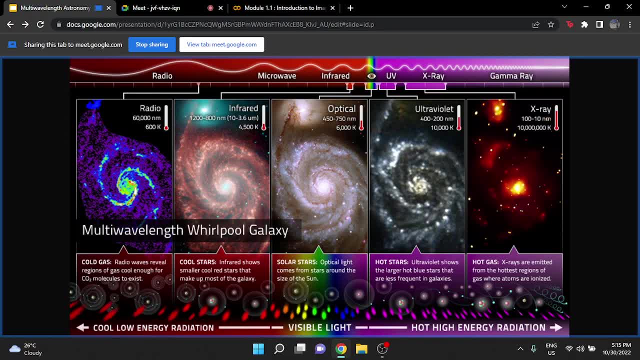 We see that we are see, we see the universe in different colors, and by colors I mean we see different phenomenons and different physical mechanisms occurring at different wavelengths. So this sort of tells you the importance of why we should study or look at the universe and if possible, all wavelengths, because if you have done basic atomic and molecular physics you must know that different wavelengths and different radiation pattern actually correspond to very different physical processes and that could tell us a lot about the galaxies, tell our population, metallicity, the star formation, history, everything. 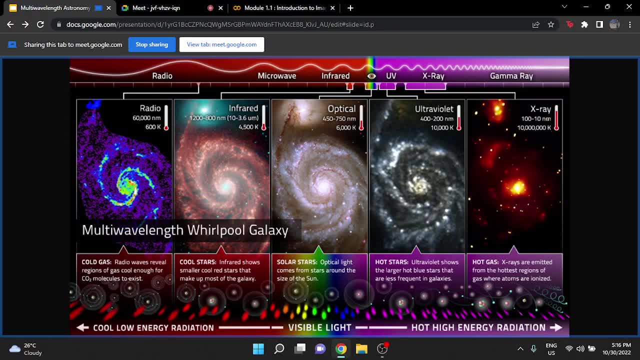 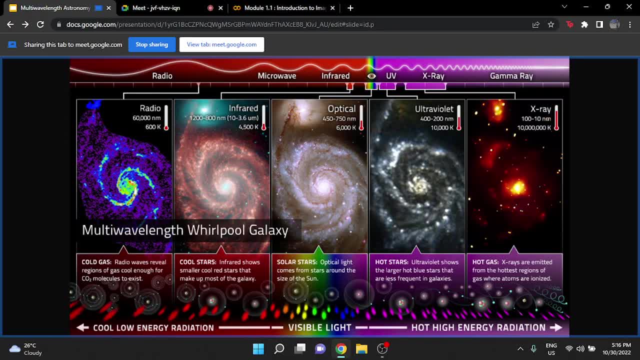 So in the module you actually made the optical image using the Serbian system survey, to which we'll be coming later. but now, focusing on the multiosing, the astronomers aspect of it, we see that we see some bluish tint. but when we look at the x-ray image, we see a totally different shape. 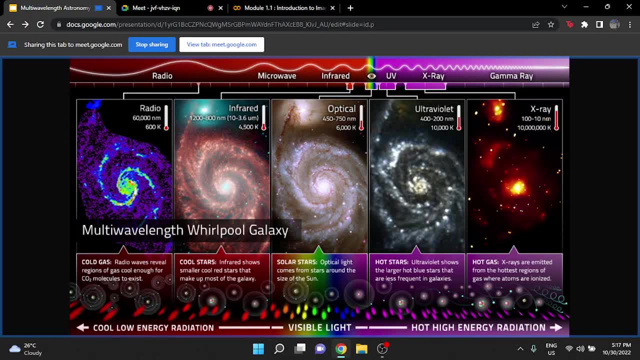 so whenever in the throughout the lecture, when i say, when i use the word morphology, it effectively means shape. you don't have to think deep there. so we see that in all the images the morphology of the galaxy is very different, and it's interesting to understand that each image 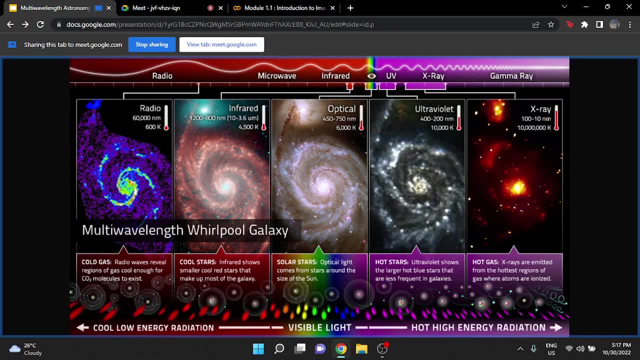 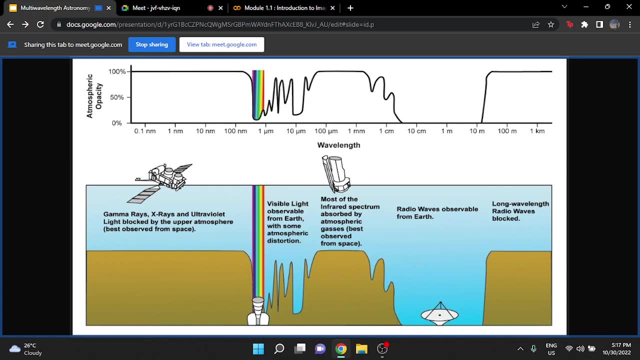 each image corresponds to a very different physical phenomenon, and in this lecture we try to like just briefly understand some of the mechanisms that are involved in each band. now the question is: why are we not exactly able to look at the entire electromagnetic spectrum from the earth? so it's because of the earth's atmosphere. 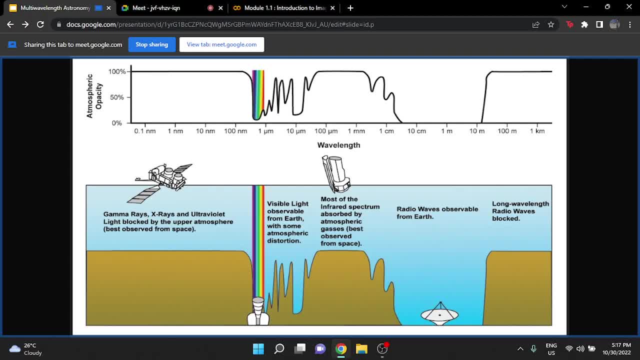 we have very small windows, pockets in the electromagnetic spectrum where we can look out through the atmosphere and we will be able to actually be able to observe something. So you must be familiar that we do not get a lot of UV rays and that is why we do not get cancer that easily, because sun's 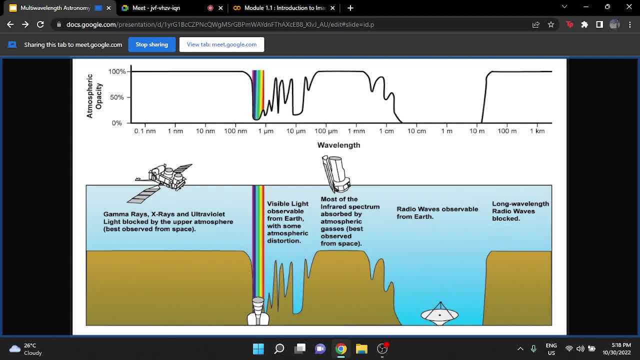 ultraviolet radiation gets absorbed by atmosphere. So even though it is an advantage in some cases, but in astronomical cases it is not that good. So in the figure you see that in the top you have atmospheric opacity versus wavelength plot and opacity is generally, if it is sort of like 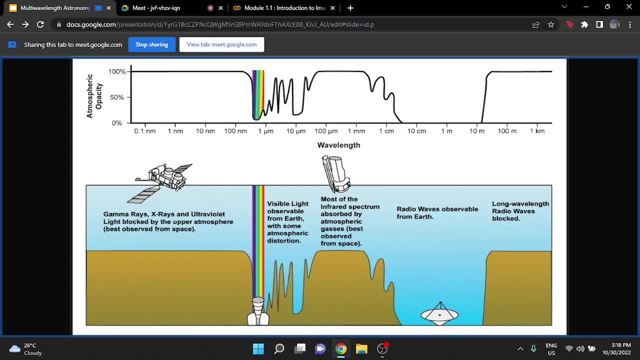 transmittance, the opposite of transmittance. If something is not very transparent, then you know it is called as opaque. So opacity is a measure of opaqueness. So we see that at the very lower wavelengths are at the lower wavelengths. So we see that at the very lower wavelengths are at 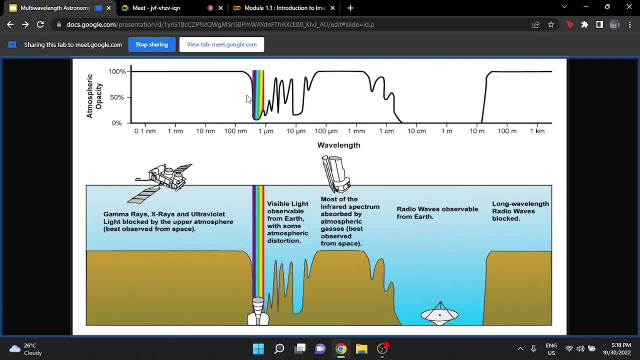 the lower wavelengths. So we see that at the very lower wavelengths are at the lower wavelengths, Atmosphere is very thick, in sense it is very opaque, and then we have the small optical window, then we have some regions of the infrared wavelengths which we can observe then right after, 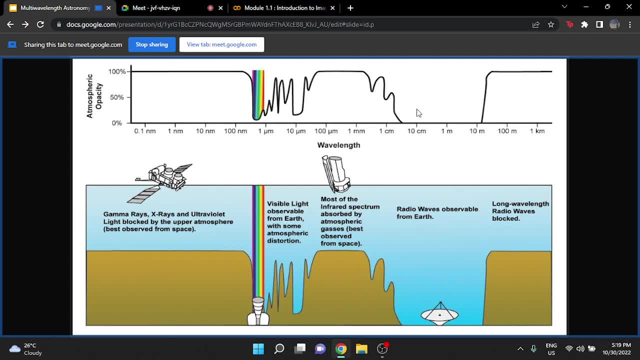 that the only window we have is the radio window, And for observing in different bands we require different technology and since some of the wavelengths are not observable from earth, we need to have space observatories. So we will actually go from left to right. that means shortest wavelengths to the longest wavelength, and looking at some of 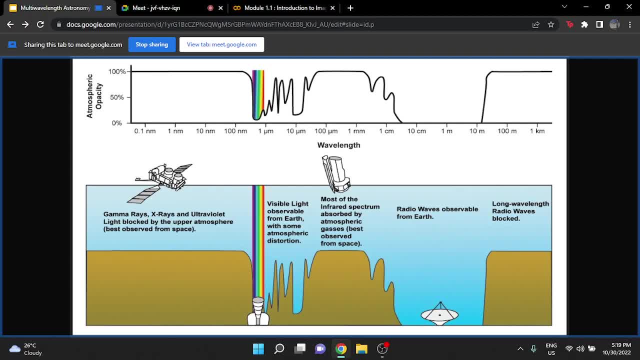 example, surveys that will be available, and this will basically make clear of all the acronyms and different names that were put in the module, And so the telescopes and surveys that I am showing you are not the most updated one, and the reason for that is for most of our projects and exercises. 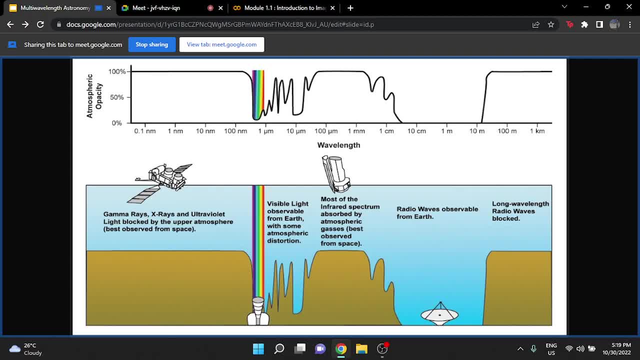 we will be using something called as the archival data, So whenever scientists observe or give a proposal, they have proprietary right over the data for a set amount of period- It could be three months, six months or one year. After that it is released to the public for that, so that everybody can use that data. So such data gets. 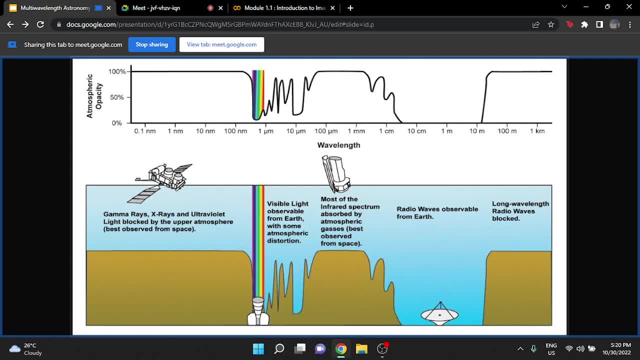 collected and accumulated in repositories and that can be used for something called as archival data things. So it's interesting to know. in the last decade, more than 60 percent of the signs actually came out of archival data signs rather than proprietary data. so to understand and know what all archival data is available. 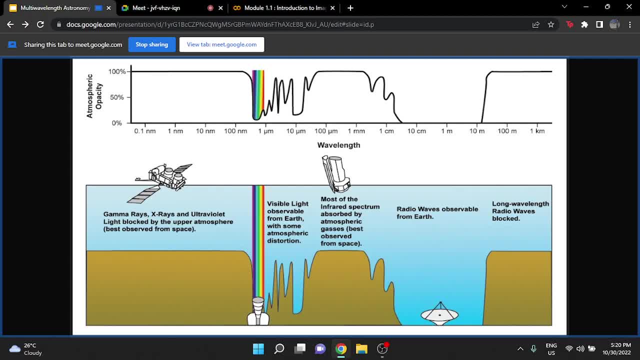 and how to access it is very important. so the first week module, as it is named, acquisition and visualization, teaches you how to acquire data using a particular mode. it's called it's, the server is called as nasa skyview, and you are using some sort of api to make these connections. 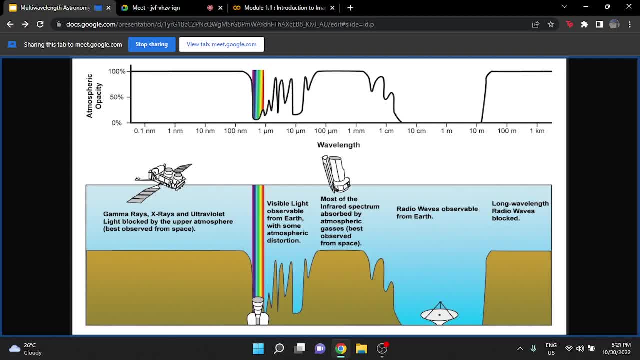 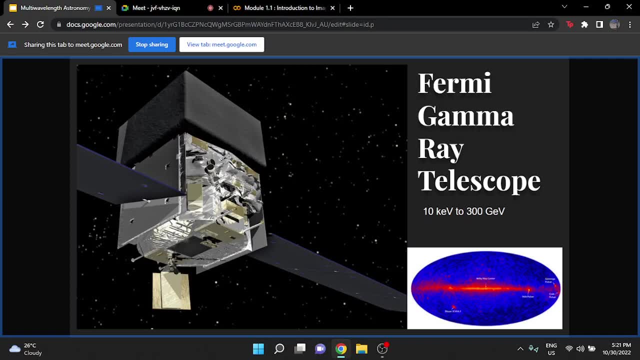 to all these, the nasa skyview server. so let's go to the first telescope, so the gamma. the first telescope is the gamma ray telescope. so the it's sort of an artistic rendition of the fermi gamma ray telescope and and the on the bottom right corner you see the all sky. uh, it's basically the. 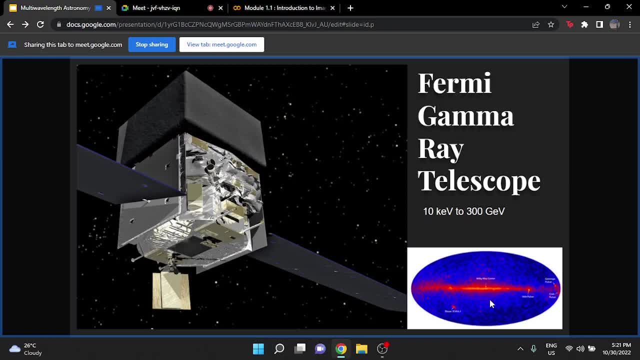 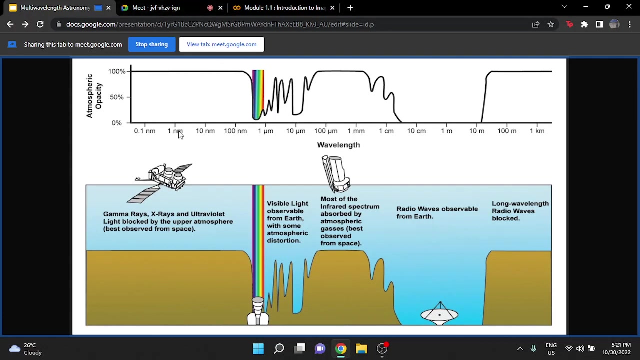 2d projection of the entire sky and this sort of gives us what this uh- gamma sky looks like in the gamma ray. hello, yeah, your voice was breaking when you were talking about archival data. okay, okay, sure, so, uh, uh, i'll, yeah, so whenever a scientist makes a proposal, 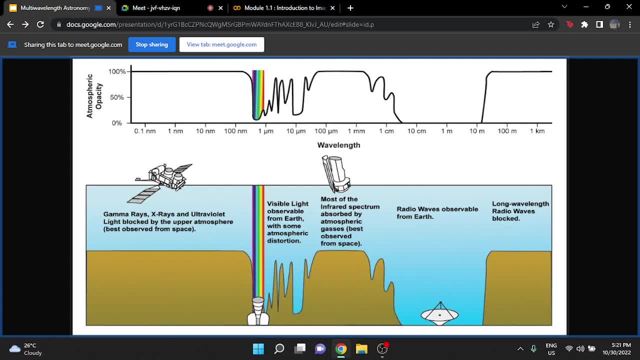 like like they'll have something called as the proprietary period. it's the duration of the period where this data is only available to the scientist to propose the project and after that period, that data is made available to the public to explore. so this is because, uh, you might be observing a particular source for your 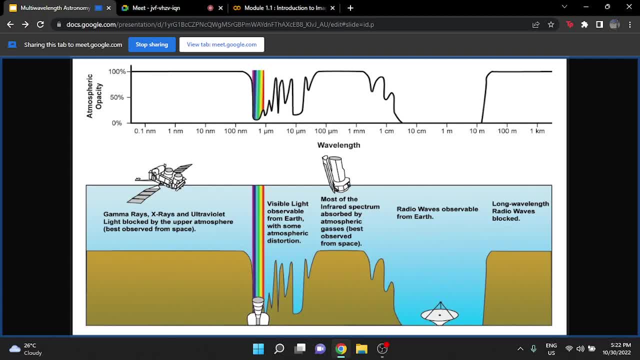 science objective, but that same observation can be used by somebody else for a different science objective. so what happens is uh, since astronomy has progressed from uh normal eye view to looking at the telescope and drawing, to ccd cameras, to digitized data, to large databases of data, these proprietary datas have been made available. 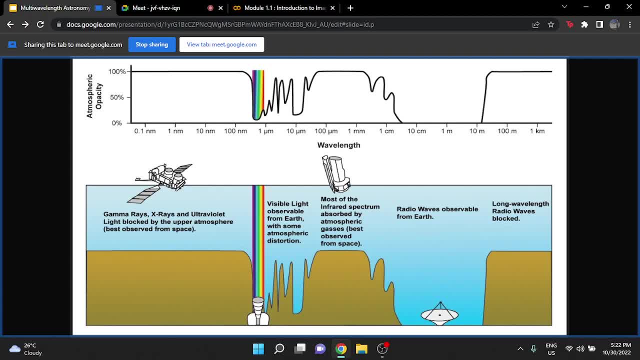 through different archives. so the one archival data that you all have explored, knowing or unknowingly, in the first module is the nasa skyview repository, and the astro query is sort of like a wrapper which accesses this skyview server, and there are actually multiple ways to. 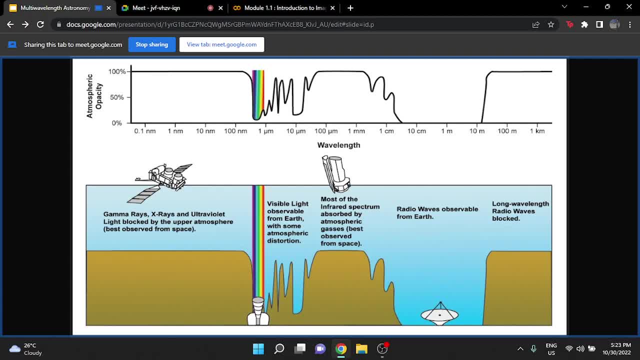 like access these archival data, but doing it in a scripted programming module sort of lets you automate a lot of processes, so, uh, the one other aspect i was talking about, archival data- is in the past decade more than 60 percent of the signs that was reported and published came out of archival 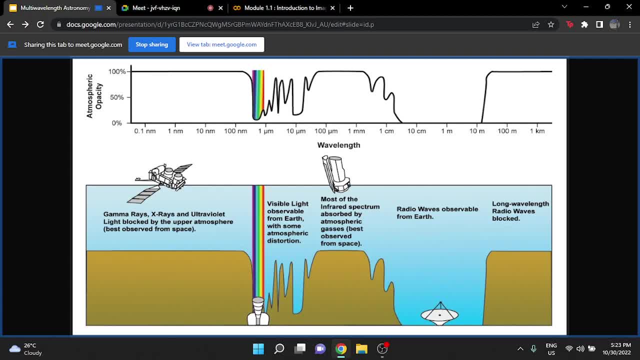 data than repos uh like proprietary data. so it's important to know how to acquire uh and how to use archival data. so that's what we looked at in the first module, which is why it is named acquisition and visualization. so uh, is that clear? shall i move ahead? 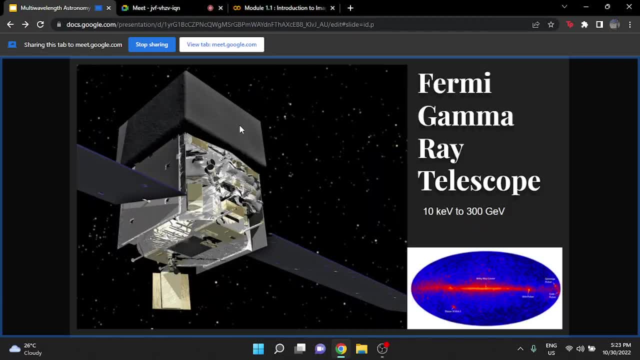 yeah, yeah. so the first telescope is the fermi gamma ray telescope, and the image that you see is an artistic rendition, and on the bottom right corner we see a 2d projection of the 3d sky that the fermi gamma ray telescope observed. so i'll tell you one more. 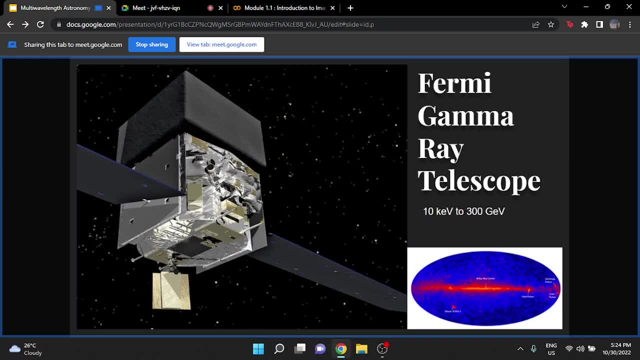 features about these observations that sometimes telescope go as something called a survey mode in survey mode, uh, the the telescope, irrespective of proposal, will have a during the telescope proposal project alone museum will observe the entire sky to get a wider view of a moving object. so to admit that the telescope will not be able to really record a 10 foot virtual map. 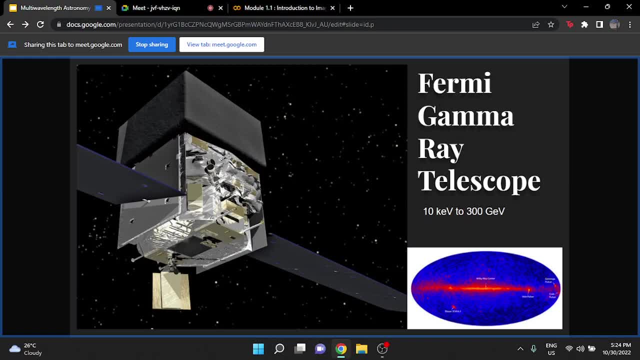 so how will it predict a real user such that when they see a 2d, gets low resolution, less sensitive survey? but this allows us to see how the sky will look in a particular wavelength using a particular telescope. so this bottom right image that you see is such an image. so this is the 2d projection, dy b 2d project, and we see this is how the telescope willunn. 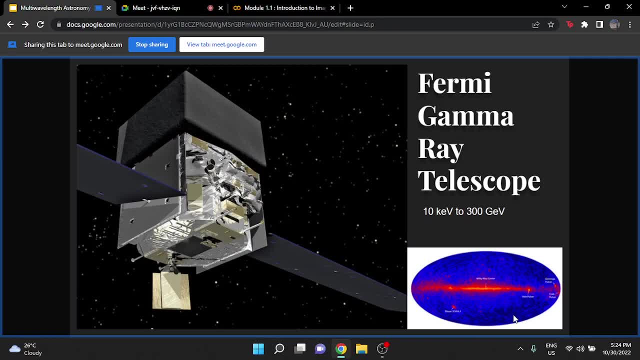 the gamma ray sky looks like. so what you see in the middle is because of the milky way galaxy or milky way. so we can't, and when we look along the milky way we only see we. we are not able to see the center nor outside, because we the the milky will still sort of obscure whatever is. 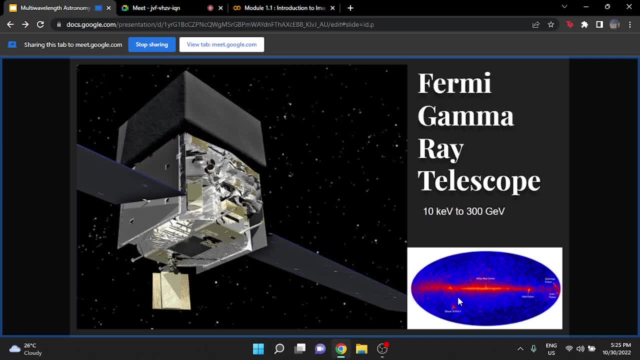 behind. so this entire sky image allows us to understand how the gamma ray sky will look like. and, on a side note, this particular telescope- fermi telescope- looks at energies: 10 kilo electron volt to 300 giga electron volts, moving on. so this is the chandra. 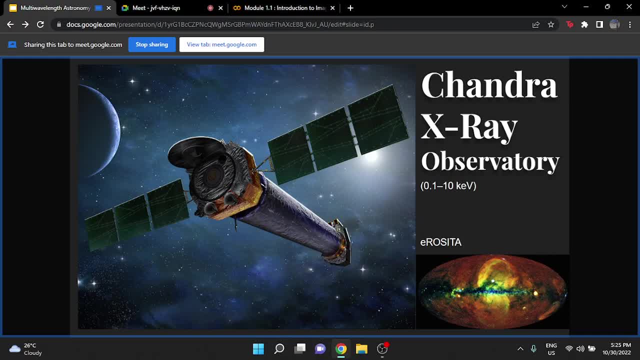 x-ray observatory and this is sort of a very popular mission and it has quite a lot of history. so chandra x-ray observatory, as its name suggests, observes in the x-ray domain and observes in the wavelength 0.1 to 10 kilo electron volts. so, as you must be knowing, gamma. 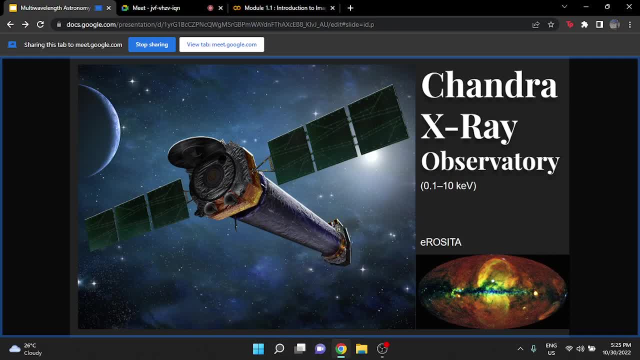 ray and x-rays have very high energy density as electromagnetic radiation and often are seen as signs of high energy processes such as like x-ray jets or hot gas or star forming regions. so, if you know from your basic optics lessons, there is a resolving power equation which is as: 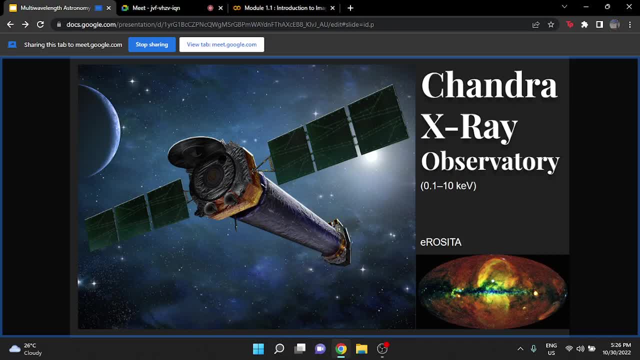 the resolving power of a particular telescope is 1.22 times the lambda, which is the wavelength the telescope is observing, divided by the size of the aperture. so this essentially tells you that the resolving power, which is basically the smallest angular separation the telescope can differentiate, is directly proportional to the wavelength, so smaller the wavelength, higher will be the 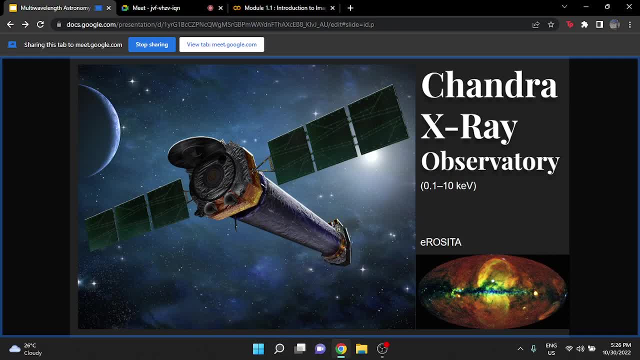 angular resolution. that means you will be able to resolve two small angles much better, if you observe it. higher frequency, so x-ray and gamma ray, sort of that's why gives really high resolution images, even if the telescope aperture, which is the diameter of the optical, the primary mirror. 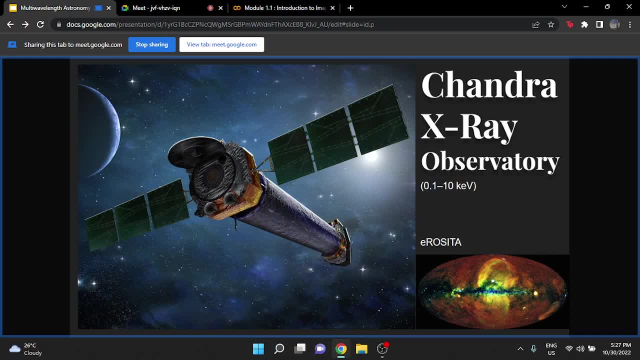 is, even if it's not big, you can get really good resolution. so, uh. so chandra x-ray observatory as a such didn't do an all-sky survey, so but erosita, which is another x-ray observatory, it did do a all-sky survey, and in the bottom right i have shown the all sky, sorry, the the 2d projection. 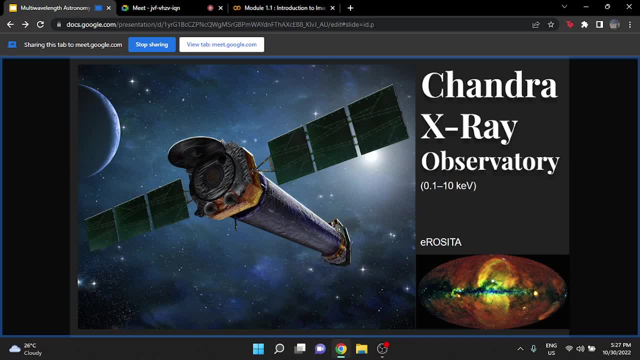 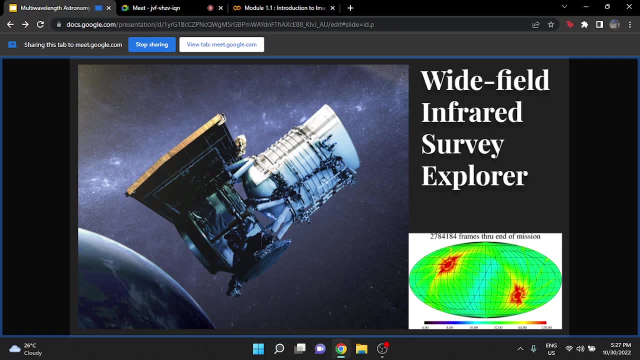 of the x-ray sky, uh, on the bottom right. so moving to the next. so next we have uh infrared, so this i have sort of uh missed out the what do you say? the order here, for another reason that this is: these are all uh, these are all old telescopes. 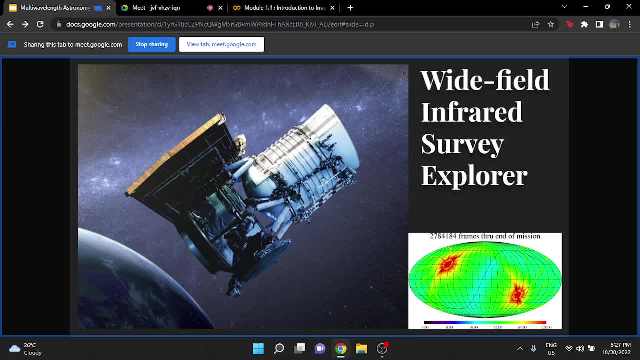 so i sort of put them together. so the wise telescope, which stands for wide field infrared survey explorer, looks at the infrared part of the sky and it actually has multiple bands like 22 and 12 micron, 4.3 micron, 3.6 micron, and all these wavelengths have very high significance. 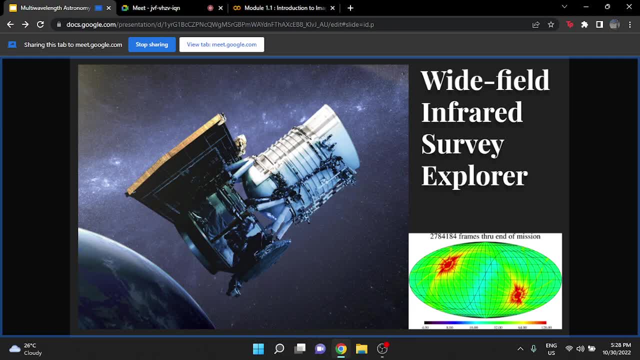 in the astronomical perspective. so whenever an observation is a telescope is planned and designed, a lot of theoretical feedback goes into its design. so at some point, like i'll discuss about the how, like what sort of work is being done from the indian side towards such multi-wave like the observatories and space telescopes. but as of now, weiss is a telescope. 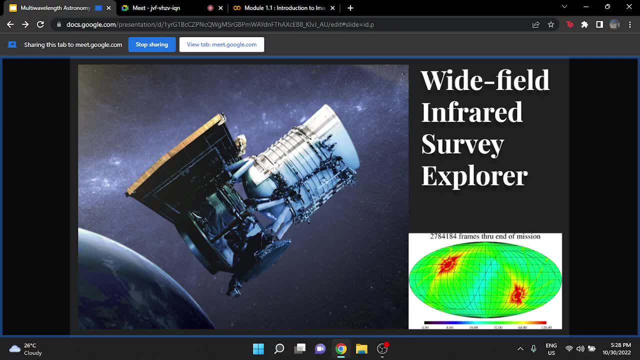 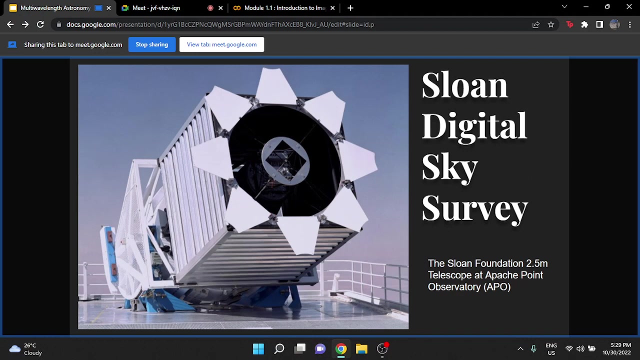 which gave us a lot of insights on like uh ir re-emissions, and it also discovered quite a bit of exoplanets and brown dwarfs. so weiss is a very important survey and it also has an all-sky, publicly available data through nasa skyway. so next we have the sbss survey. so this is one data. 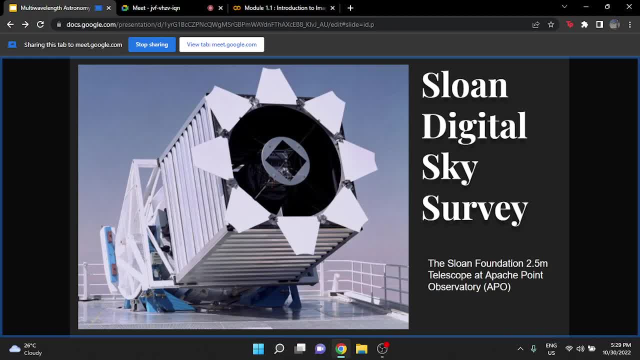 that you actually used in your modules. so sdss stands for the slow and digital sky survey. it uses the 2.5 meter slow and foundation telescope at apache point observatory. so this particular telescope is very important in our course because we'll be using many different. 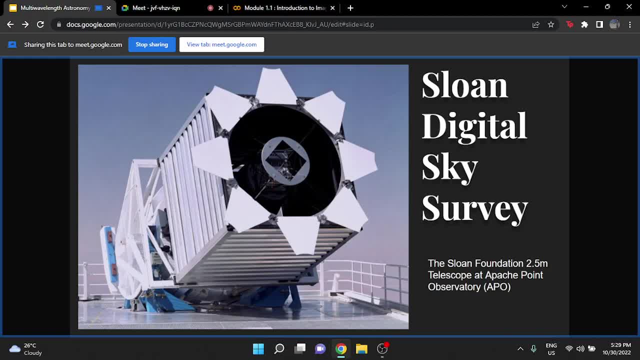 surveys and results that this particular telescope got. so a lot of scaling relations that we use in astronomy was actually in the last decade was made possible by the sbss survey. so weiss is a very important data that was made possible by the sdss telescope. for example, whenever we have scaling, 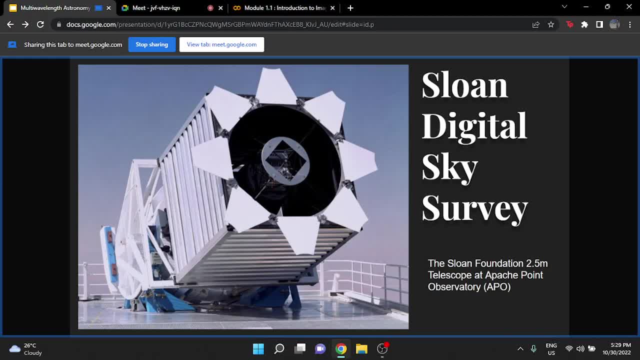 relations for, say, the star formation rate or the specific star formation rate. it's okay even if you don't understand these jargons, but essentially what i'm trying to say is a lot of data in spectroscopic and imaging wise was made possible through the sdss telescope and we'll be using 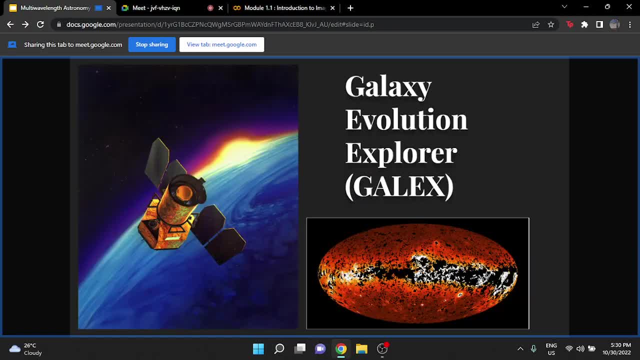 quite a bit of it in in our entire course. so this is the galaxy evolution explorer. it stands for galaxy, which is actually galaxy, and it looks at the uv part of the sky, and it mainly has two bands, which is the nuv band and the fuv band. 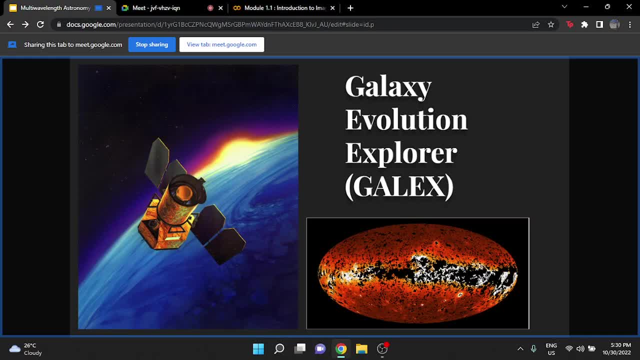 so galaxy actually has not that greater resolution, but it did have an all sky survey which allowed us to look at a lot of uh? uv, counterparts of the optical galaxies and the optical phenomena, you know, phenomenons that you see. so, uh, i see that it's 5, 30.. uh, so, and we have actually covered. 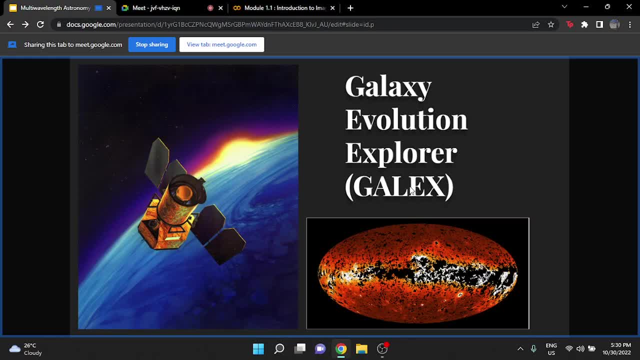 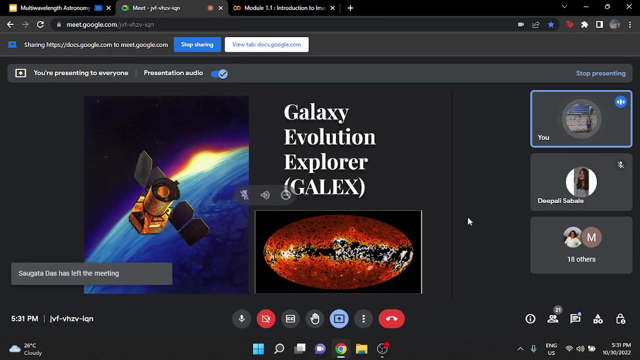 one major section of our course, uh, the lecture today. so, uh, if you guys want, we can take a break for five minutes. if you want a break, just drop a yes in the chat, or if you don't want a five minute break, you can drop a no. 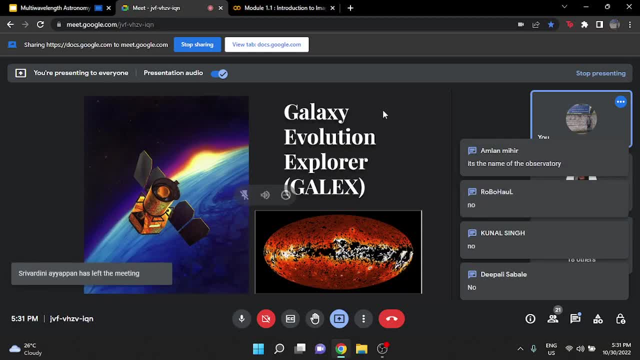 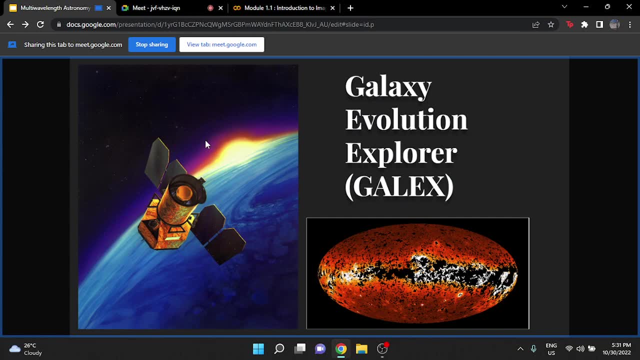 yeah, good, so the galaxy evolution explorer is the, the particular observe, the telescope. it also is available in nasa skyview and you can use it to locate the uv counterparts, which actually tells you about energetic processes such as star formation, asian accretion or mergers. 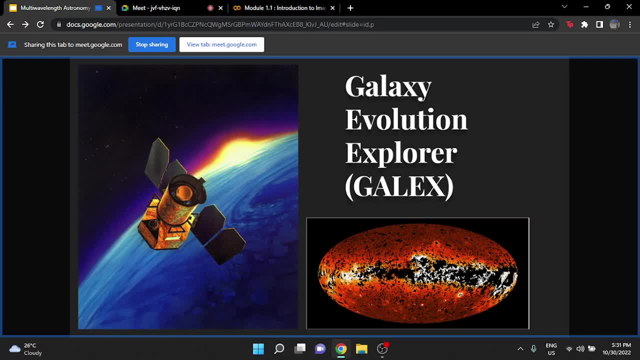 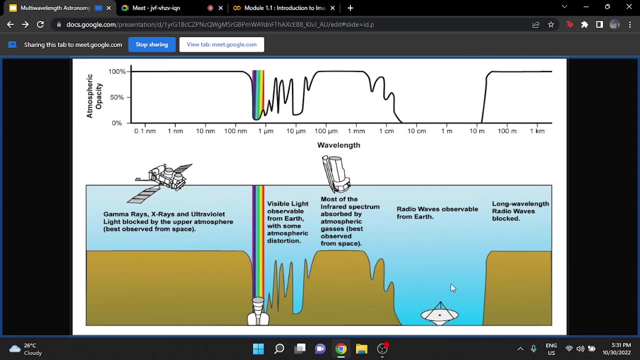 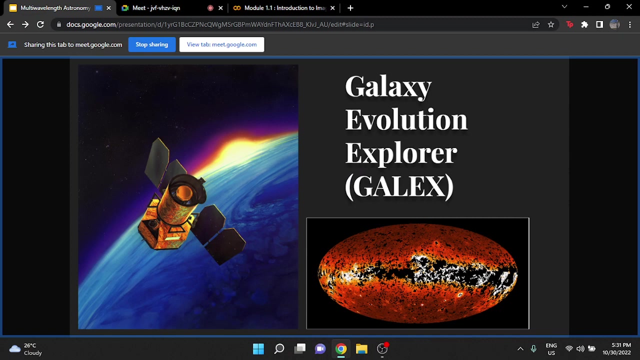 so these are the some telescopes and some surveys that we'll be actually using in our multi-wavelength observations. but apart from this, as i showed in the initial, there's also the radio wave observations. in this particular presentation i haven't included much of radio observations because the physical mechanisms that are actually explored using radio surveys. 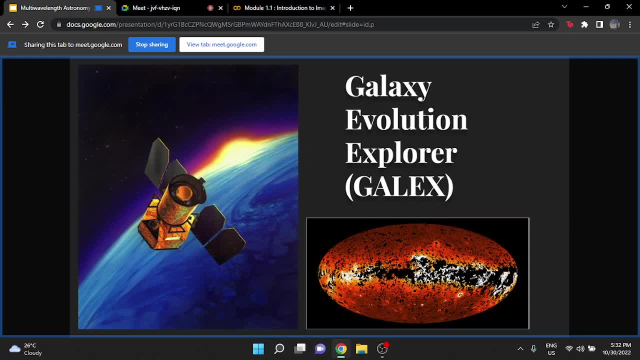 is as quite, uh, physically like the. the physical mechanism that undergoes is a bit difficult to grass and i didn't want to confuse you at this stage, but if at a later point, if a lot of you are interested, we can even explore radio astronomy and radio astrophysics. 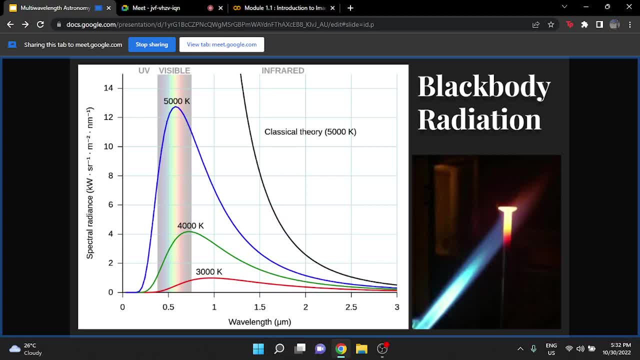 so now that we understand some of the telescopes that are available and where they are now, we can look at what sort of information can actually be gathered from the image analysis or image procurement you did. So I believe all of you must be knowing blackbody radiation, and we know this one key feature. 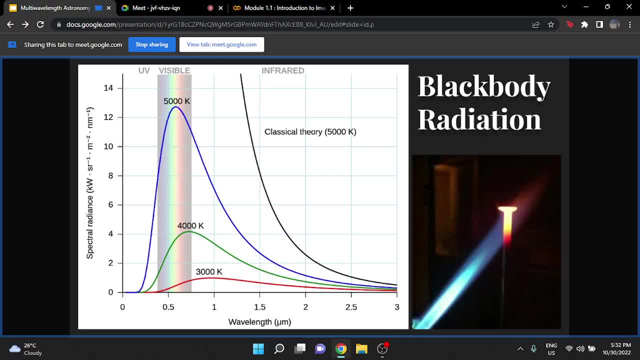 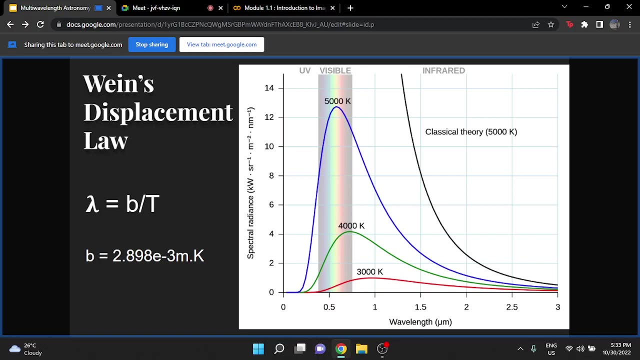 of blackbody radiation is that it depends on the temperature. So for each temperature there is a unique blackbody curve. So if you remember, from the blackbody radiation derivations there is one approximation which is called as vane's approximation, and it gives you a law called the vane's displacement. 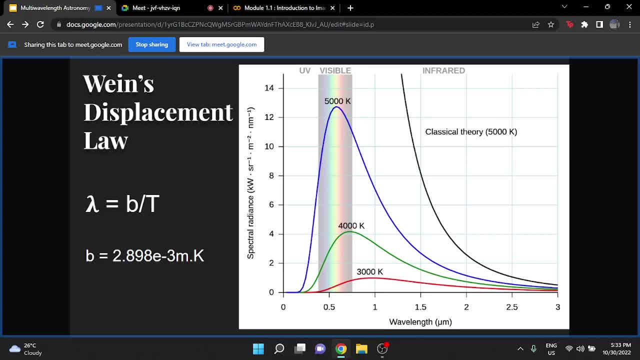 law which gives you the proportionality relation between the peak wavelength and the corresponding blackbody temperature. That means for a blackbody, if you know what wavelength it is peaking at, that means you can give its corresponding temperature. So this is actually very useful. 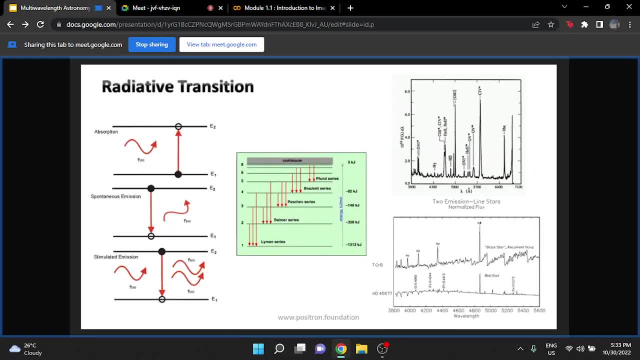 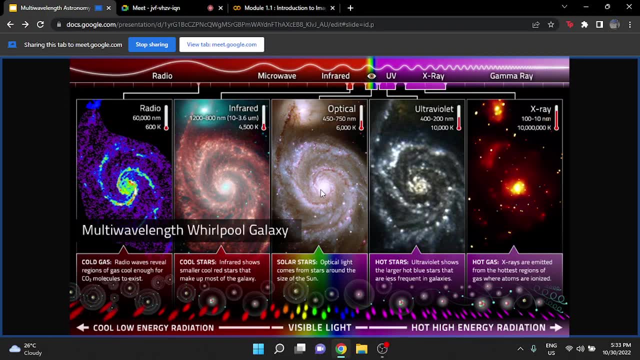 This will result when you're doing multi-wavelength observations, and I'll try to show you how. So imagine you are looking at the optical image. You're looking at the optical image and you know what is the wavelength of the particular observation, like which wavelength that particular optical observation is shown, and from vane's. 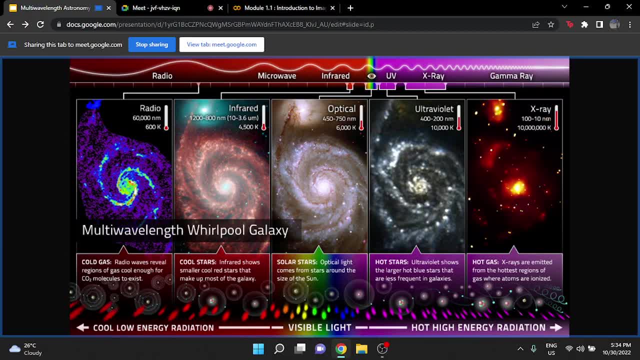 displacement law, You can find what the corresponding temperature is to that particular wavelength. Now, assuming that what you're seeing is undergoing the blackbody mechanism, we can find out what the temperature is. So, for example, say you're looking at the blue, you see that there's a lot of blue part. 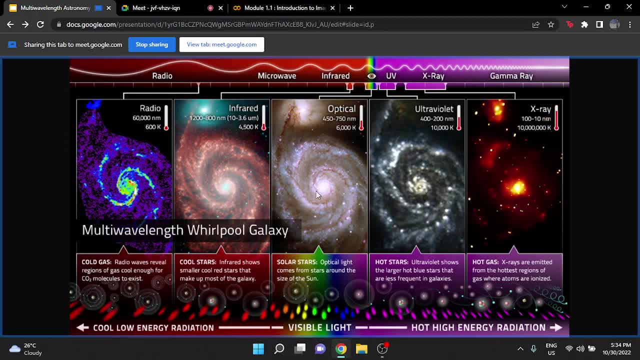 in the image, and this particular image is RGB image. but we'll come back to what RGB image is a bit later. But using vane's law, what you can do is, if you know the peak wavelength, you can find out the temperature. 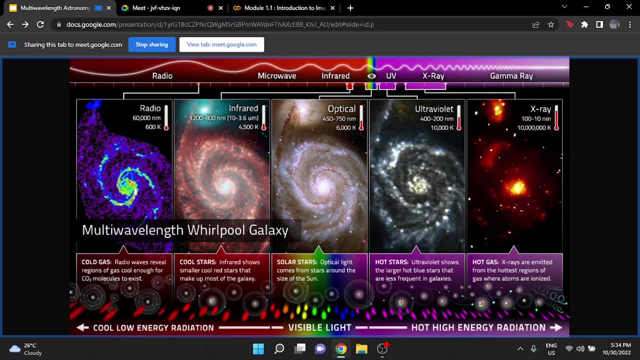 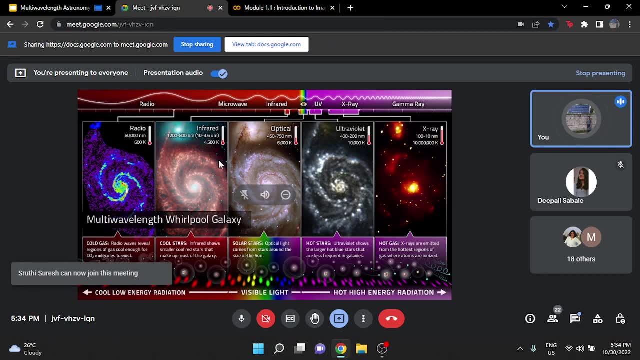 So for now, I want you to just remember this and keep in your mind that if you know the peak wavelength, you can find the temperature. Okay, Given the key assumption that it's the radiation mechanism is blackbody radiation mechanism, But we know that blackbody radiation mechanism. 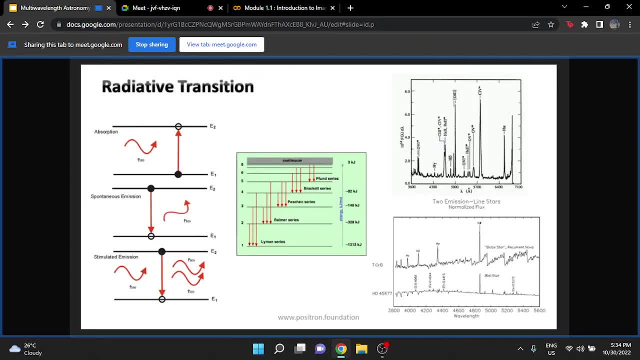 Okay, Okay, Okay Okay. It's not the only way to get radiation. There are a lot of physical processes which can have give rise to radiation, So we have radiative transfers. I'm not going to go individually into each of these processes, because each require one. 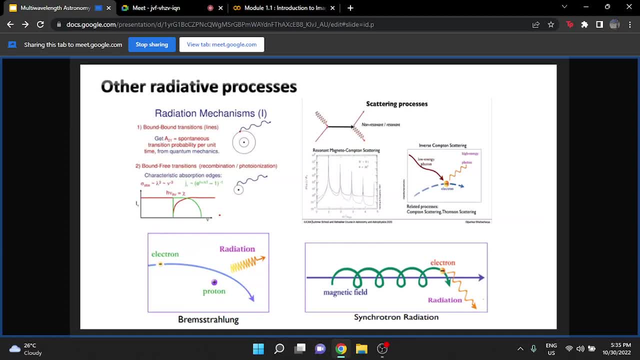 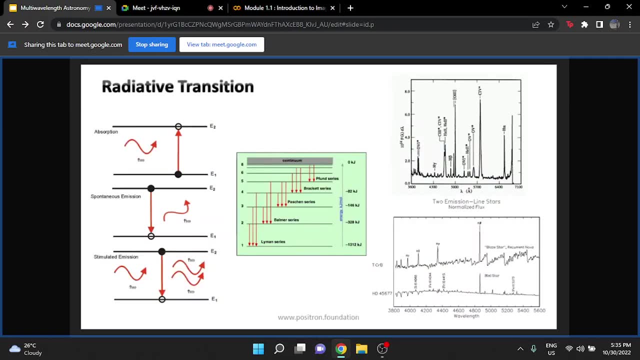 course, But in generally we know that there are many processes So we can get emission lines from. take this: quantum radiative jumps like absorption emission. all these processes could happen. We can also have processes like Bramstrehler, Okay. 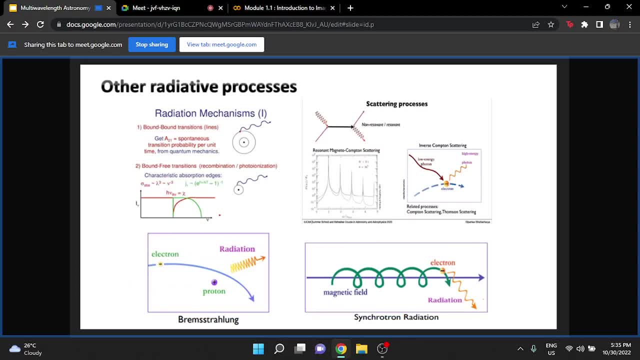 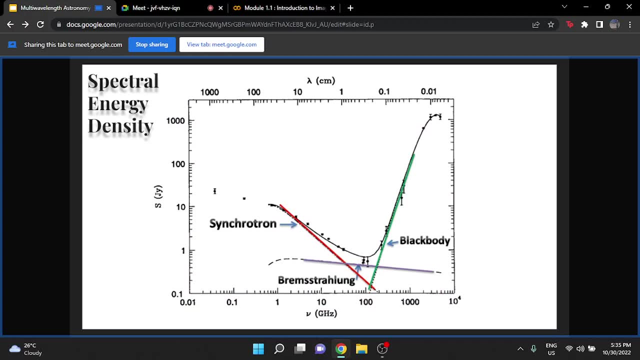 or synchrotron radiation, based on the physical situation of the, where the emission is coming from and what we essentially get because of multi-wavelength astronomy is: see now, from a single wavelength you can only find out if the mechanism which is causing the emission, if it is blackbody. if it is not true in other cases, for example, if it is synchrotron or 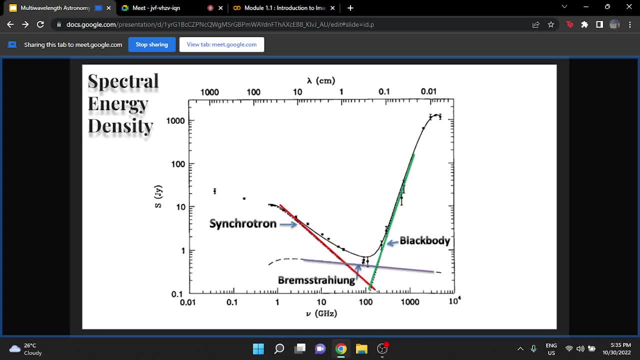 bramström, sort of an emission process or radiation process. you need observation at multiple wavelengths to make something like what is shown in the slide. so this is called a spectral energy density diagram. so here we have flux versus the frequency. so what tells you the radiation? 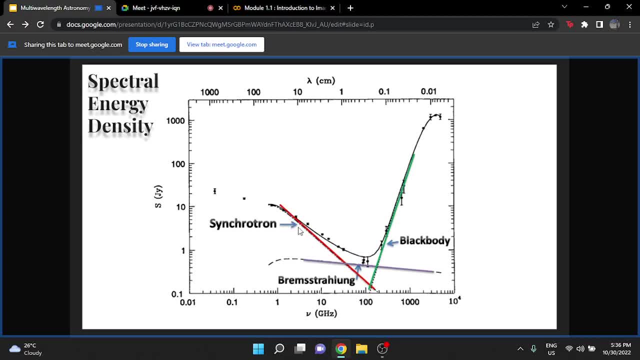 mechanism is where it falls, what sort of slope the radiation has. so the slope tells you what sort of physical process is causing the radiation that you observe. and one interesting feature that you see is there are points where the radiation could be because of multiple processes. so you 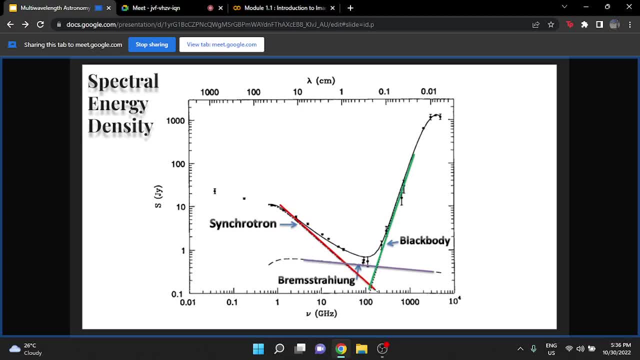 can't simply actually say just based on the wavelength that it is, this is the temperature. so if you know that synchrotron and bramström radiation are non-thermal radiation, that means they have no temperature correlations directly. so this is the synchrotron. 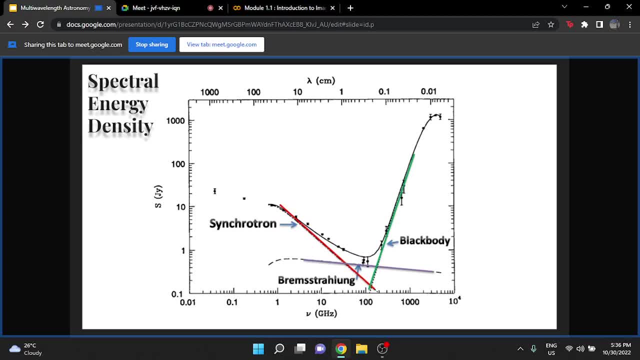 radiation is what fuels most of radio astronomy and it's a bit theoretically involved. so maybe at a later lecture we'll go a bit more depth on synchrotron radiation and how do we observe it and what sort of projects can be pursued using the data that we have. so 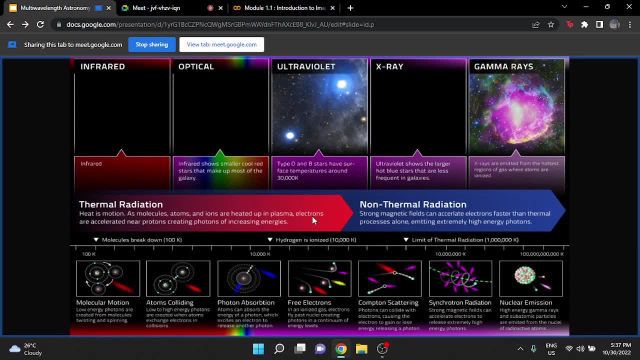 now, as i said, like a lot of observations that we and a lot of exercises that we did, we did using either ir or optical or, in some cases, cases uv data, and to most extent most of them do come in thermal radiation, so you can use vane's displacement law to say what the corresponding temperature is. but now, when it, 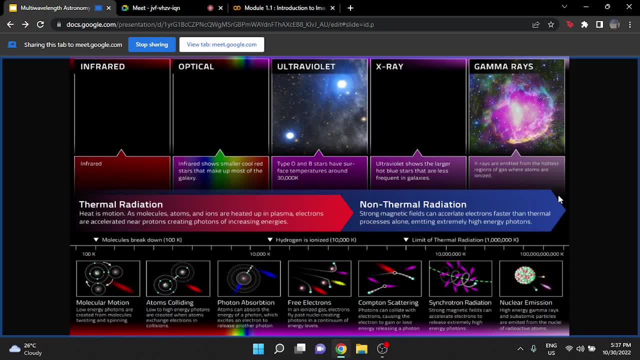 comes to x-ray, gamma rays and even including radio, you can't exactly do that. so that's why, if we include that also, our problems becomes way more complex, because then we'll have to do these scd fitting and spectral index analysis. so that's above the what's aimed for this course, but so far 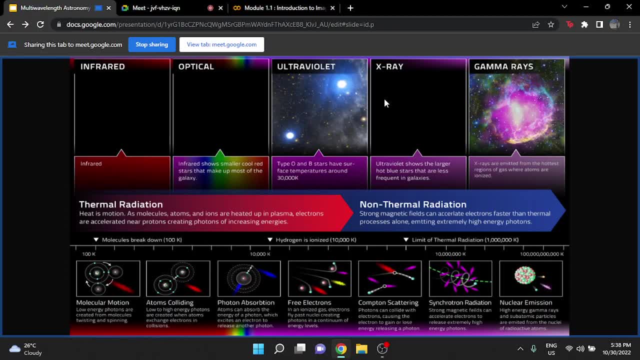 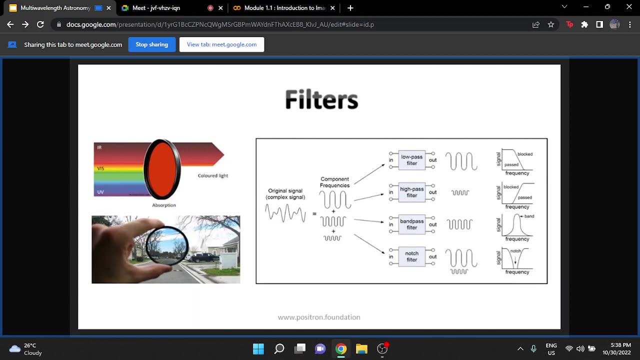 the our analysis till the course project, let's limit our study to infrared, optical and ultraviolet radiation and thus those sort of data. so in the exercises you must have seen this word being used again and again, which is filters. so stss has these many filters, so essentially it is very similar to the filters that we come across in our 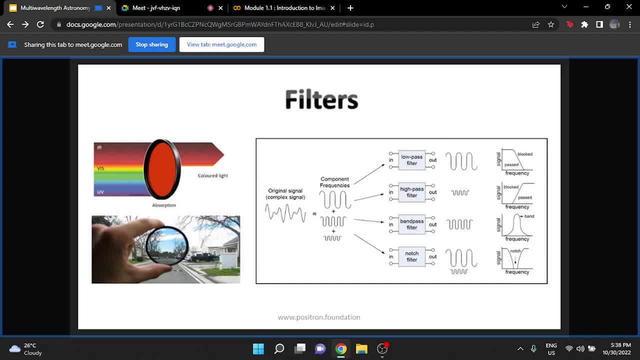 electronics class, where we have low pass filter filter, high pass filter, band pass filter, band block filter. so we know that and i think most of us understand this. essentially what it does is it removes or keeps a particular section of the radiation that we're getting. so in electronics we 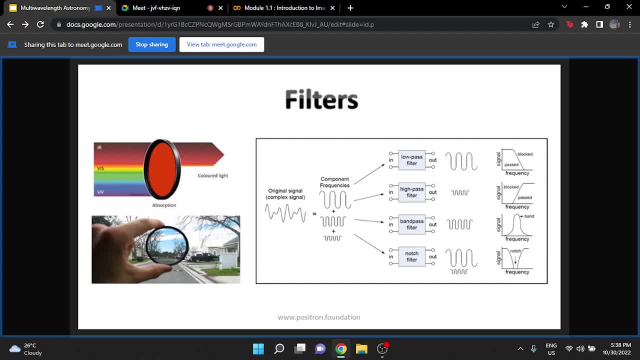 do this with frequencies. if we want to do this with frequencies, we do this with frequencies. if we want to limit, we only want: from this frequency to this frequency we keep a band pass filter so we get radiation or we only get oscillations in that particular frequency. 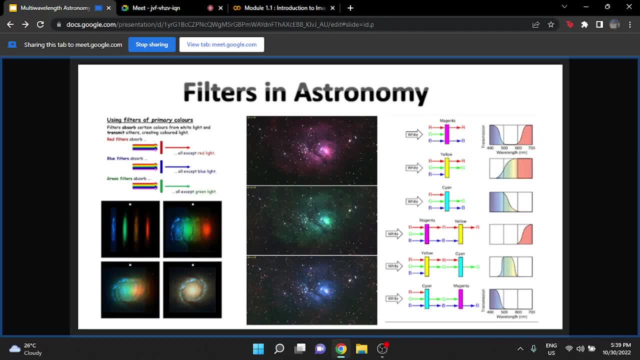 so very similar to that. there are filters in astronomy where we try to get specific sections of the electromagnetic spectrum, as each give us very different information, as we understood from the multi-wavelength astronomy brief diagram. so each wavelength filter will tell you a bit different information. so from very basic blackbody radiation study, we 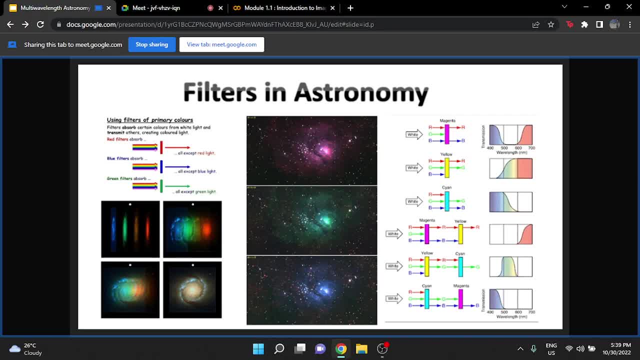 understand that red has a higher wavelength and blue has a lower wavelength. so, applying that logic to vane's displacement, if something is blue, that means it has a high frequency, that is low wavelength, that means it has high temperature. so i'll sort of apply that logic to vane's displacement. again, we know that red has a higher wavelength, green second, 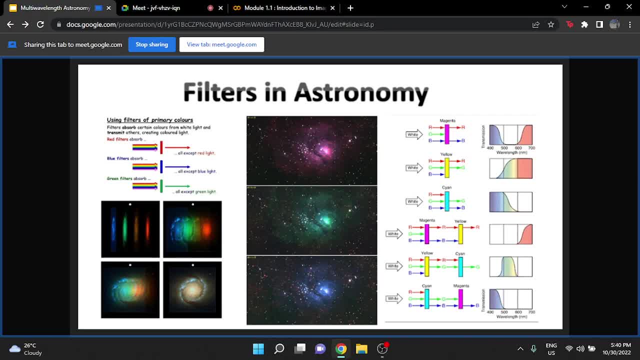 then blue has the smallest wavelength amongst visible rgb colors. so right now i'm talking about visible red, visible blue and visible green. this will be important the later stage. so now, if we apply the vane's displacement law, blue, since it has the shortest wavelength, it will have the highest. 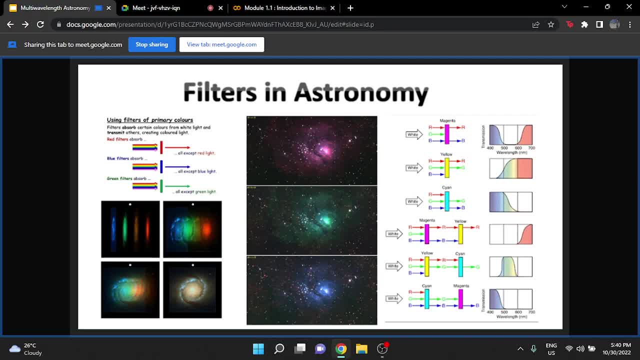 temperature. similarly, this exact logic amongst rgb t, amongst rgb red, will have the relatively lowest temperature. so whenever you look at an image and you know it is giving you visible rgb colors and you see something as blue, you know that it it has higher temperature. now we'll try to. 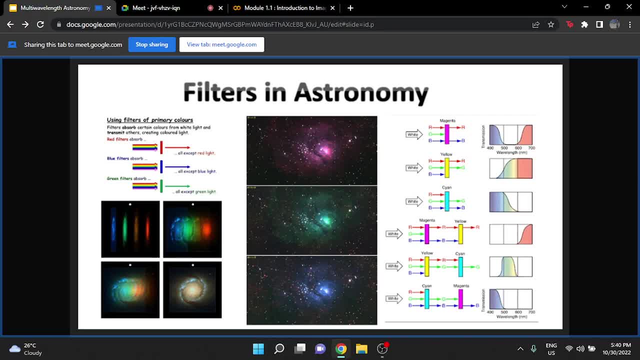 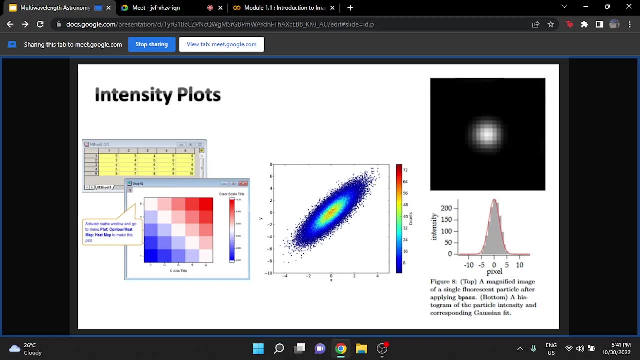 make this understanding and make this concept more clear. so let's go ahead and start with the concept like root in our mind a bit more deeply through couple of examples. so yeah, first let's start by understanding: what do you exactly see when you make an image? so the very first thing. 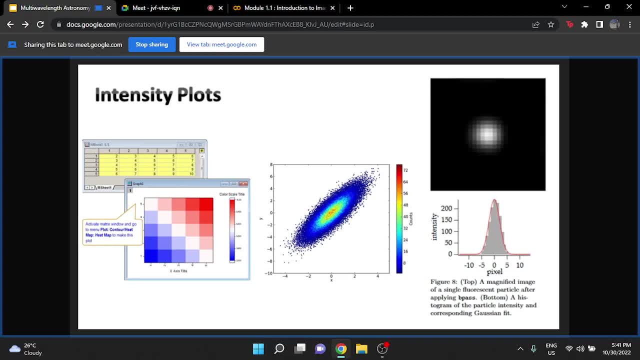 that you did in the exercise was to make use the fits data and make plot the image. so if you look at the image you'll essentially see. if you have seen the array, it is basically a 2d matrix of different numbers And what you plot is basically the relative intensity or the relative 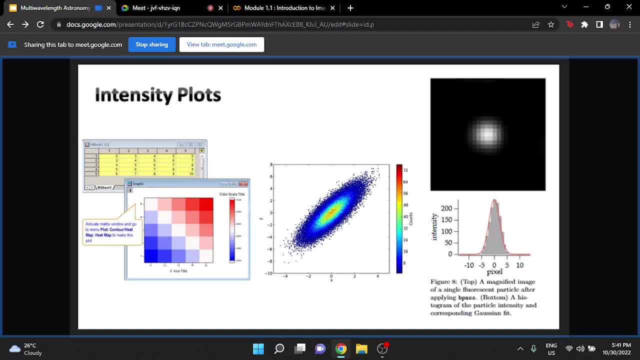 amplitude of each positions in the 2D matrix. So such plots are called as intensity plots, And this is not only used in astronomy to any way where we have a parametric field which has three parameters. We often use the put two parameters in the coordinate axis and we put 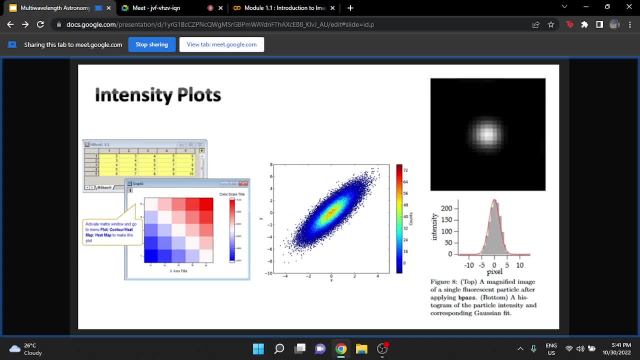 the third parameter in the color axis. So when you are looking at a galaxy image, you are essentially looking at position versus brightness. So you are getting for each position what is the brightness that you are getting. So this is called as intensity plots. Now, from the very first slide, 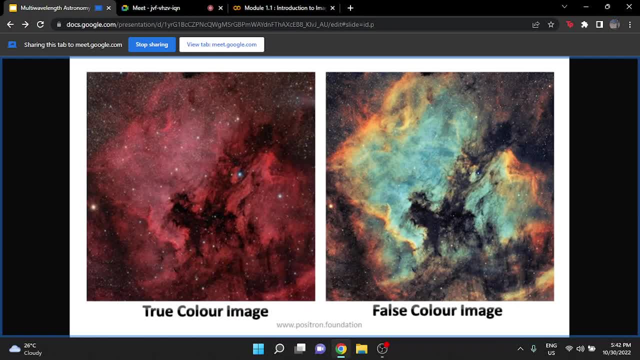 that I showed you. we know that we can only see the visible part of the sky. So how do you see x-ray UV images if our human eyes can't capture them? We can't capture those wavelengths because we are limited that way. So here is where this one. 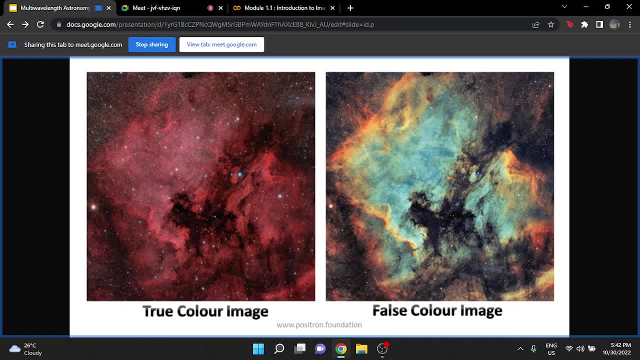 astronomical technique comes called as false color imaging, And I believe a lot of you must have faced this issue, that why are we putting red in blue when we have a red filter? So what is the convention is, since we can't see UV or IR radio, we assign a color that we can see. So, say you. 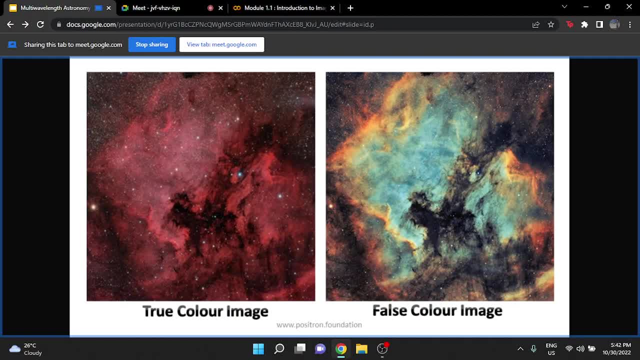 have a galaxy. you can't see x-rays, So when you do the observations, what you have is numbers. So all of you have used different color maps while you were making the images using matplotlib- So very similar to that. you assign a color to each number, because what you essentially have is a 2D. 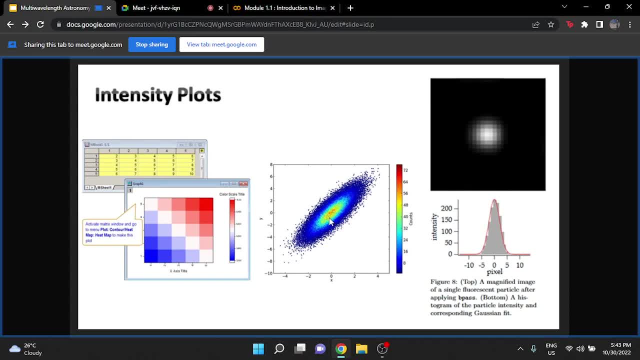 distribution like this, with the third axis of amplitude. So what you do is you assign a color for each number. So what you do is you assign a color for each number. So what you do is you assign a color for each amplitude. You'll say that if it is zero, it will be black, If it is one, it will be. 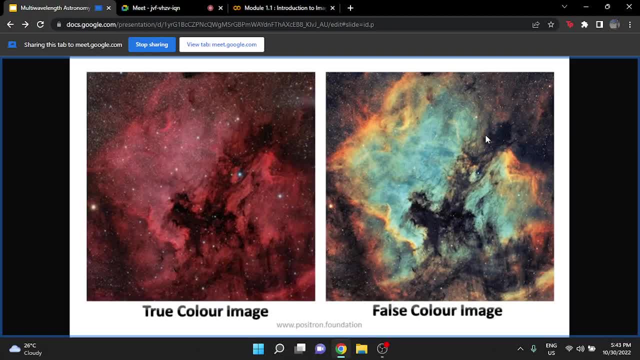 white. So you're sort of giving a color map. So most of the pretty astronomy pictures that you see, if you went in real life and looked at those it won't look that pretty at all. So those things are called actually true color images, which is all the colors that they use are transcribed into. 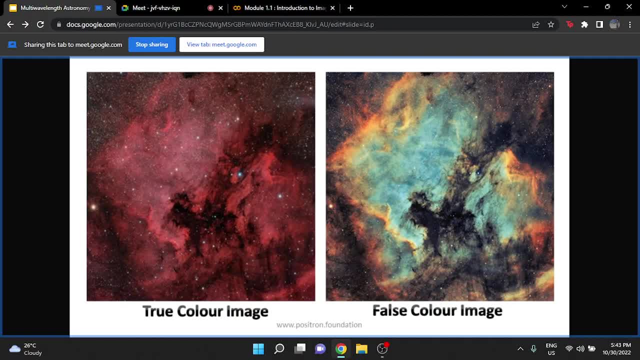 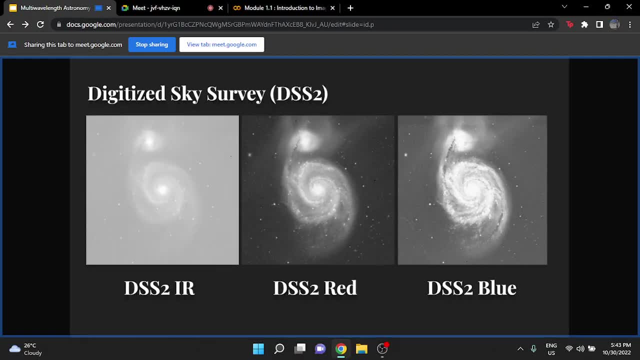 the colors which are how human eyes would actually perceive. So most of the astronomy images are called true color images. So most of the astronomy images are called true color images. So most of the astronomy images that we see are such false color images. So let's do a small see a. 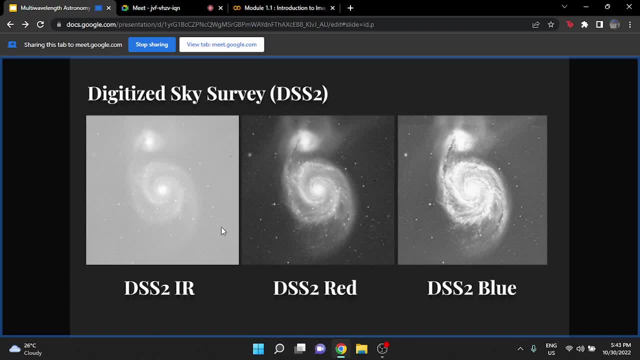 small example, again using the whirlpool galaxy, And this is the very first RGB image you all must have made. So the processes that are given to make these images are simply routines. So they don't have any explanation and they don't require, because that is just a method to see. So if you 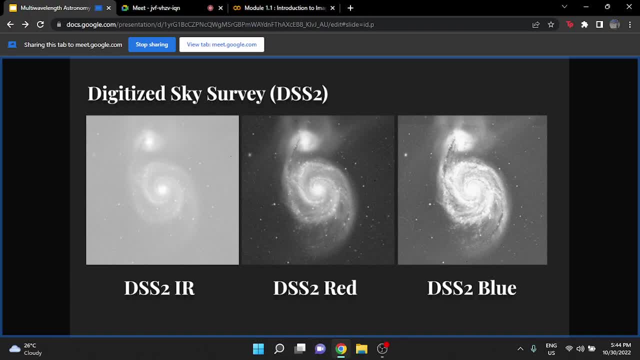 when you go for different methods, there'll be different routines. So it is essentially like learning a tool. So if you have a pencil, you write, you don't. you don't have to learn to write every time you get a new pencil right, So it's essentially a different pencil. 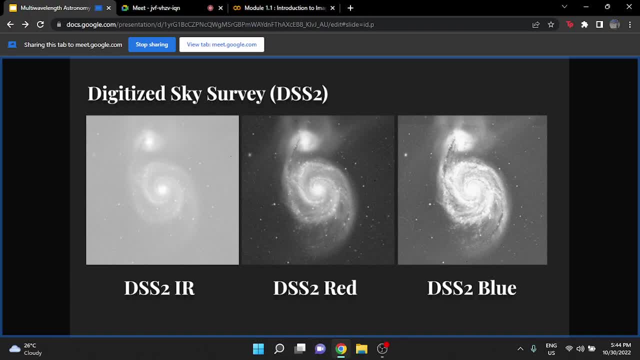 but the logic still applies. So every time you open a package, the documentation will tell you how to use it. So you won't always have to learn or watch a video how to use the package, because plenty of documentation is available. but to know what to use it for is. 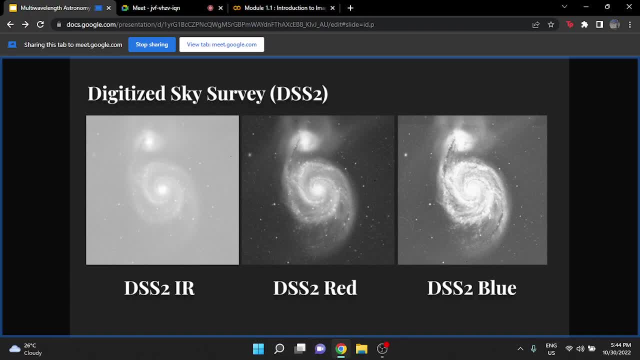 you know the you need some sort of input, and that's what we're going to do. So I have three images which I have procured from NASA Skyview. The first data is from DSS to IR, So DSS is another. 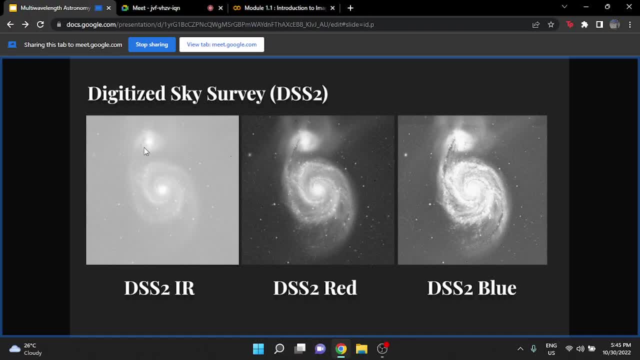 survey. It stands for digitized sky survey, So it is the digitized version of the Paloma sky survey. So this happened in the early, I think couple, 50 years ago, when we used to use this photo Metric, these plates to this photographic plates, to do astronomy. And we used to. there was a time. 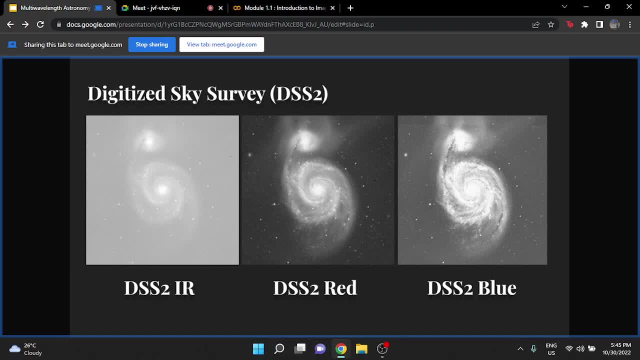 when photographic plates started degrading. So the digitized mission. what they did? they digitally scanned each of these photographic plates and digitized them. So hence the digitized sky survey. So if you actually look at in these some of the images, sometimes you will see 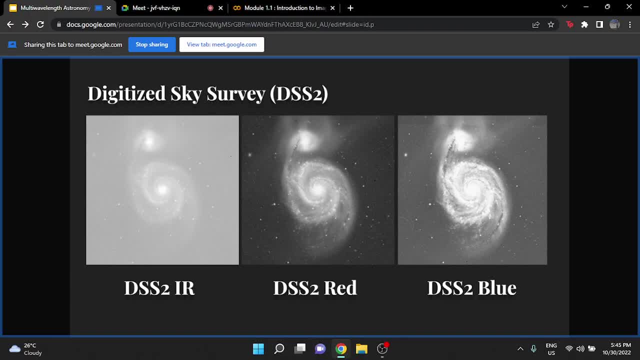 some artifacts of photographic plates. So now coming back to the topic at hand. so these are three different images of the same galaxy, observed in different wavelengths. So DSS to IR is observed in the infrared wavelengths, DSS to red corresponds to observations in the optical red and DSS to blue corresponds to the optical blue. 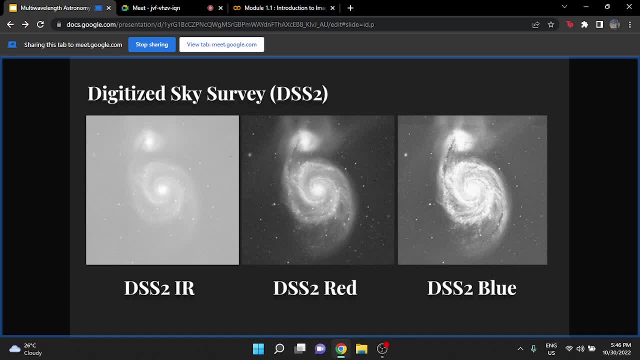 So I hope this is clear. So we have IR, optical red, optical blue. Now, since there is no meaning to color here, since IR we can't essentially see only red and blue. see, what we are going to do is we are going. 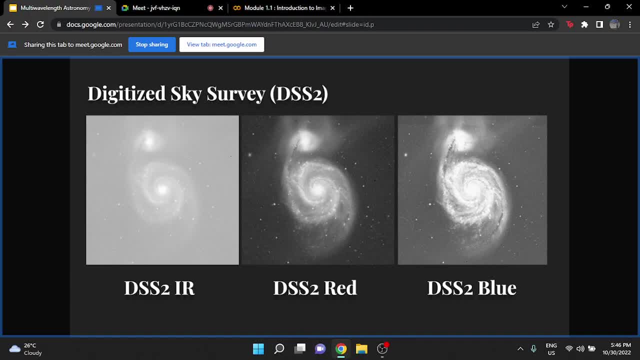 to do false color imaging, we will assign a color to each of these data. so I will assign red color to DSS, to IR. so red color means it has the highest amplitude and if it is black that it means it has the lowest amplitude. similarly, I'll assign green color to the DSS to red. so it is just a convention. 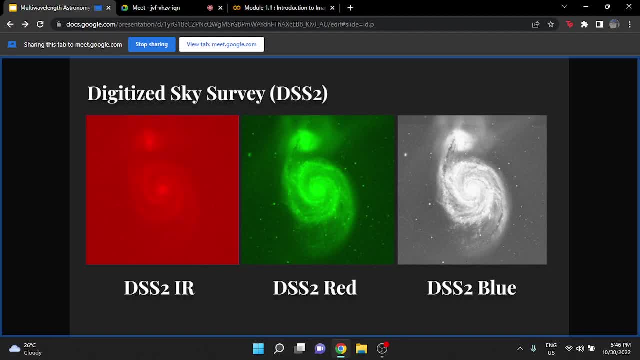 that you usually go in what you say increasing order of frequency. so the lowest frequency will be red and the highest frequency will be blue. so that is the reason you'd see that DSS to red doesn't always mean that I have to put it in red color. so, since I have put assigned the color and 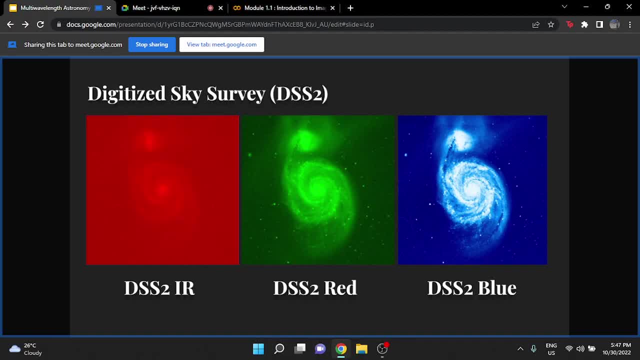 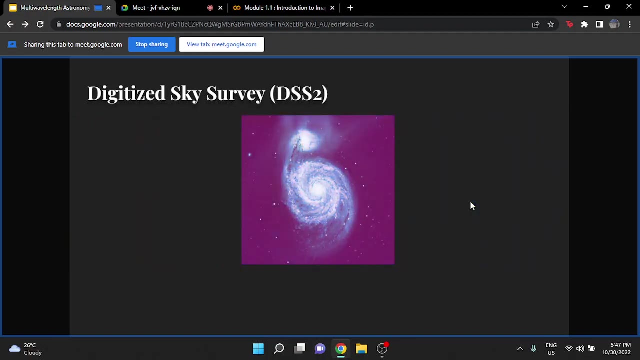 to be honest, we can put any color, any image, in any color, but there is actually a logical reason why we prefer this convention of increasing order of frequency. so now, since I have one color assigned to each, what I'll do is I'll combine the image and we will get the RGB image that we get. so now, 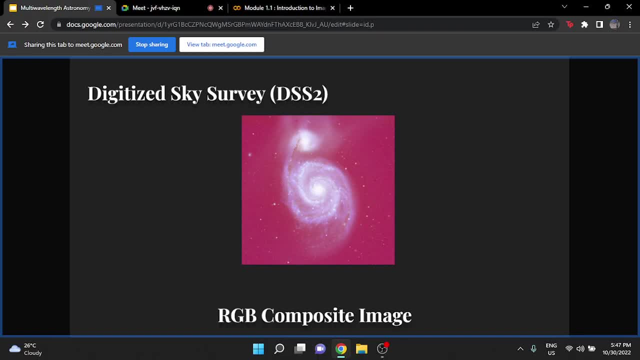 a lot of signs can be done by simply looking at this image and I, from experience, what I found is our test: make most observation from this image than physicists, because we go after there is a black hole, there is this tidal winds and there is merger. but artist can find out most. art person will first. 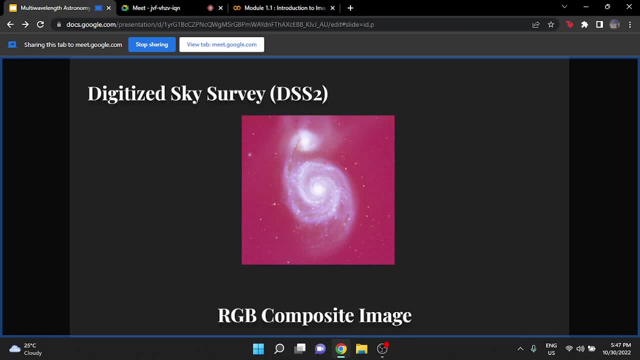 of all say it looks blue and the sort of a red hue. there are these two white smudges somewhere and there is a pretty spiral structure and that simple observation has a lot of physical consequence, for example, like when i started talking about vane's displacement. we know, we. 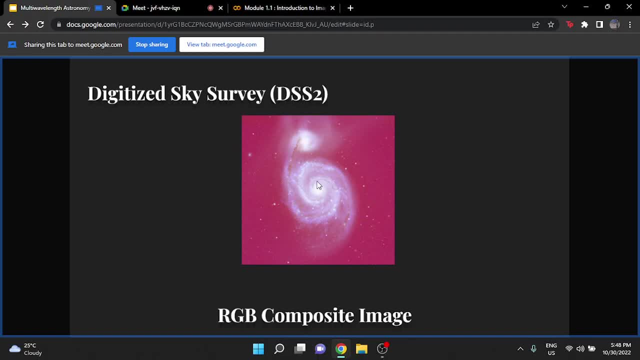 see that this particular image has lot of blueness in it. so a lot of that implies whatever we substituted in the blue filter has a lot of influence in this image. so, relatively, whatever is in the blue filter has maximum influence on this image. now, in our case, the blue filter. 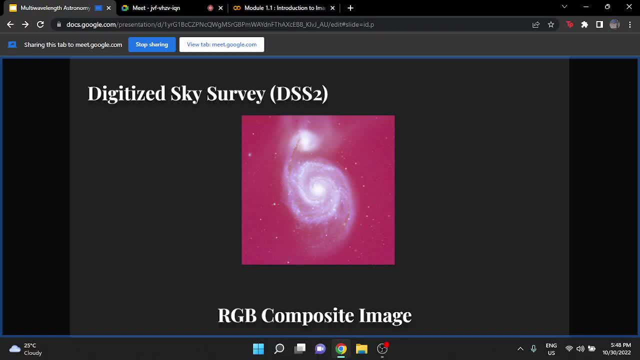 corresponds to optical blue, but that might not be true always. i could put uv in blue, i could put radio in blue, but that only means that whatever survey i have assigned to blue color is peaking. so now let's do a bit more astronomy by just looking at this image. so, since all of this, 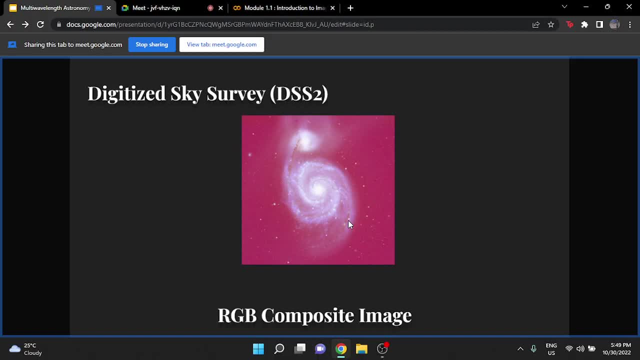 majority of the what we see in the image is blue. we can say that in using vane's displacement we can say that the blue color is peaking. so now let's do a bit more astronomy. that whatever c has we are seeing has high temperature if you actually go and substitute. 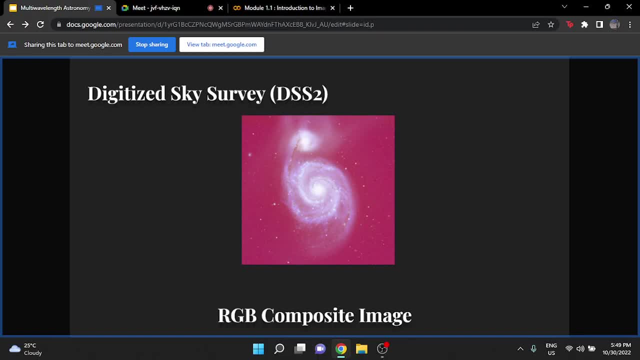 the wavelength it will come of the order of 10 000 kelvin to 15 000 kelvin. so that corresponds to very hot stars, so stars which are young. and now the opposite is what is true for red. so we see that some part of these, the spiral arm, has red obscurations. so whatever corresponds to these, 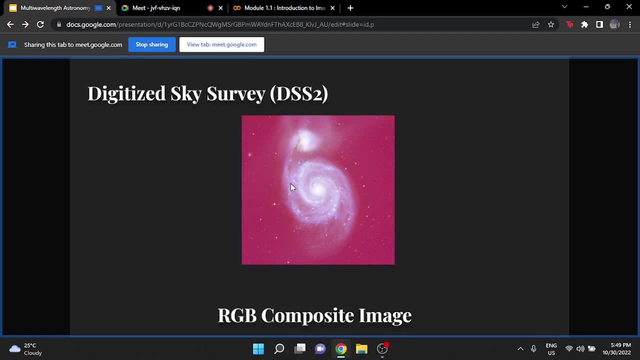 red obscurations will be the red color of the image. so we can say that the red color of the observations could either be absorptions or could correspond to stars which have lower temperature. now, at this point we can actually make a lot of physical predictions using simple physics. now we 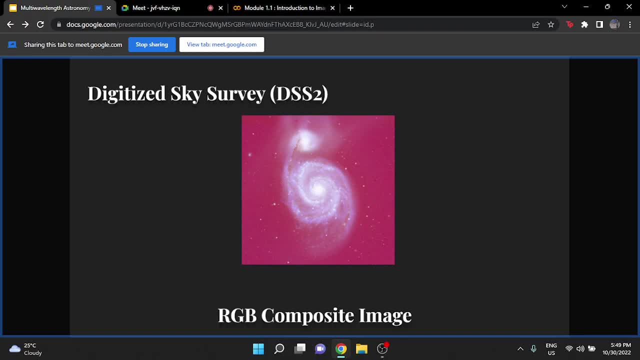 know that the energy, that any object which has, which which follows all thermodynamic laws, is limited. you only get a fixed amount of energy to do anything. so even if it's nuclear reaction, after a certain time it does run out. so if we have a fixed energy, and since these stars have higher temperature, that means they are 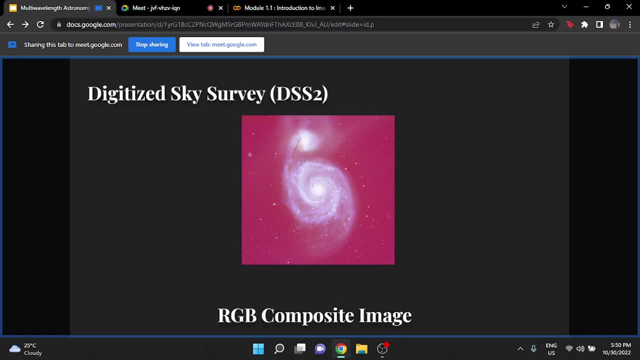 expending higher amount of energy. if you're spending more energy, extending energy more faster, that means you'll spend it in a very short time. i'll say that again. so blue stars: since they have higher temperature, they must be having higher energy output. if they have higher energy output, 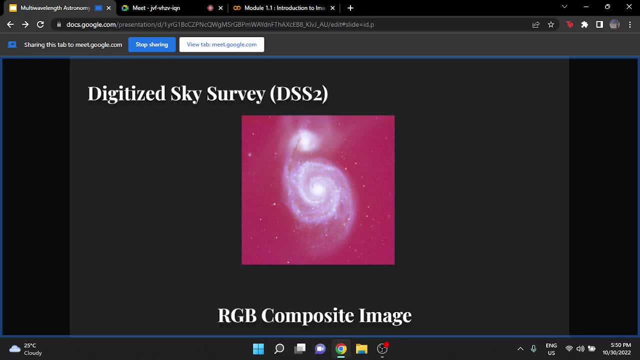 that means they must be dying fast. so all the stars that you see in blue, by this logic, are young and backtracking the same logic we can use for red: if something is spending the energy slowly, and that means it has load. if something has low temperature, it must be spending the 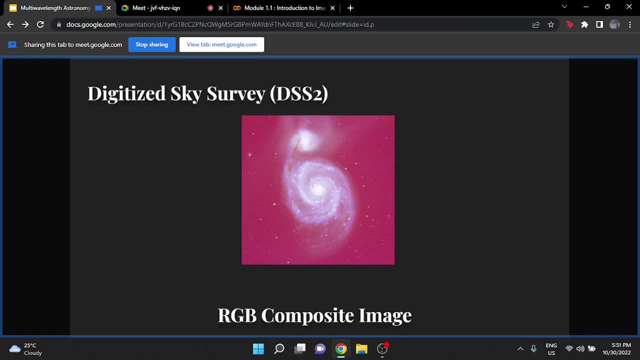 energy at a longer time, that means those stars could be older. now, with young stars, if you say that something only lives for, say, two years and you are seeing that thing there, so if you are able to see something which lives two years, that means it must have born, must have. 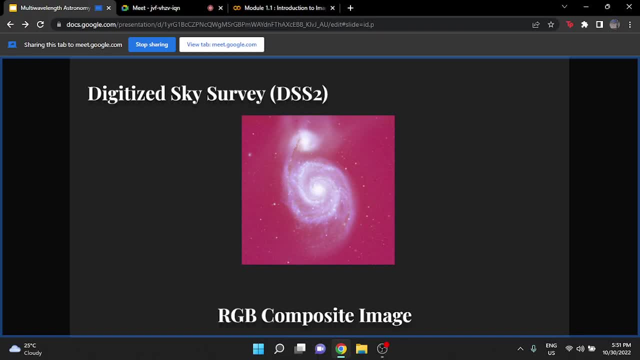 born in the last two years, that means it's young. so, basically concluding whatever i said in the last five minutes, if a star is blue, that means it has high temperature, it is massive and it is young. so if it is young, so also that if it's a high mass, that means it's a short-lived. 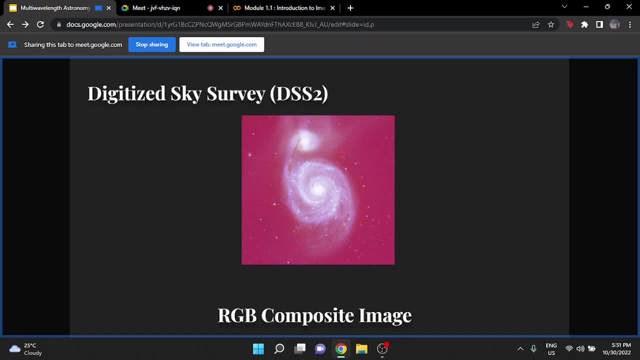 the very exact opposite works for whatever you see in red, if you're looking at optical red, if it is red, the star is low mass, older and it has a lower temperature. so by just looking at the image and knowing which color corresponds to which electromagnetic band we were able to find. 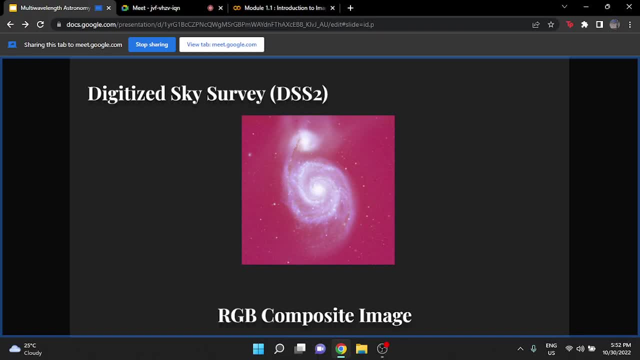 you the age of the star, the size of the star and which stellar population it corresponds to, and we see that theoretically that is very true. we do expect to see a lot of young star formation and massive stars in the star forming regions along the spiral arms. so this sort of analysis. 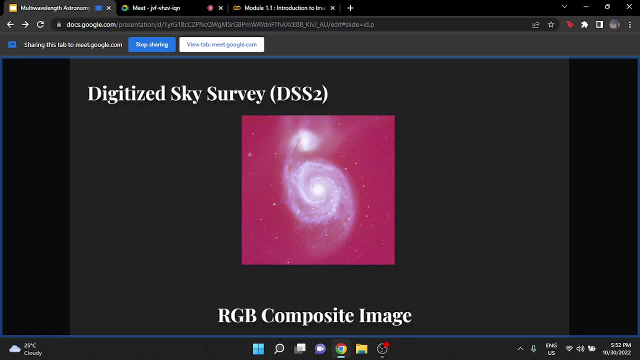 gives you a very- not a very- critical analysis, but gives you an overall analysis of the stellar population and, uh, the age of the galaxy and the mean stellar age of the galaxy. now, from the shape of it, we see that there is a spiral, arm-like structure and 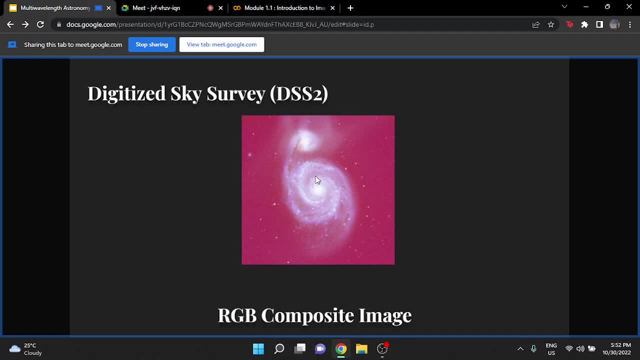 from knowing basic, basically, how wall pools work. we can see that this galaxy might be rotating in anti-clockwise direction. so it is pretty logical, right. you just have to see where the retrieving end of the spiral arm is pointing towards. so this is sort of rotating in anti-clockwise And we also see that there are two regions which are white in color. Now 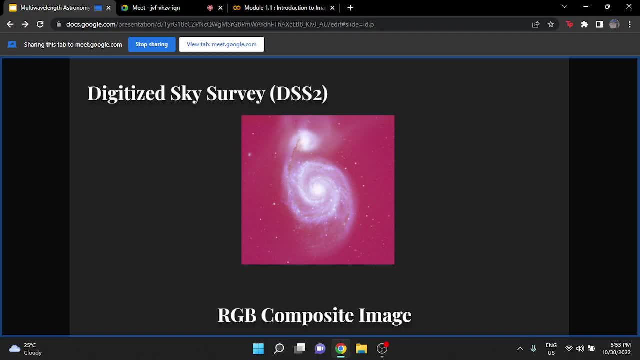 this is important. If we look at the colors which we made to use it, which is RGB, we know that we get white color when we mix red, green and blue together. So if they all have come in equal intensity, they make white. So we know that information, as whatever is in the middle is. 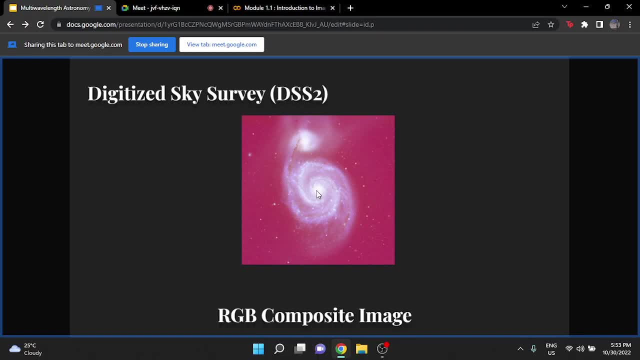 emitting almost equally in all three bands that are used. And from a sort of basic extragalactic astrophysics we know that almost all- in a sense all- the galaxies host a supermassive black hole in the middle and they are known to have such broad emissions. So that is the reason we are. 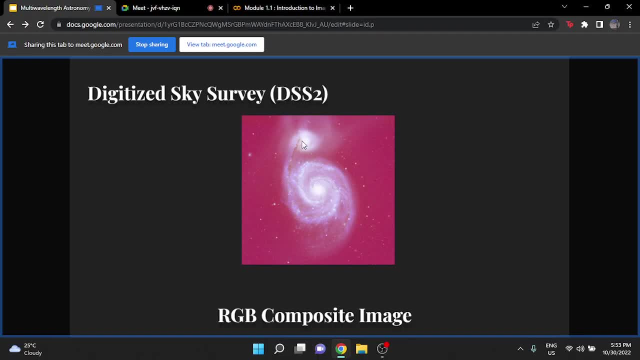 seeing white. So if this is a black hole, that means whatever emitting here must also be a black hole, which is exactly what we are seeing here. So if this is a black hole, that means whatever emitting here is exactly true. So this is Whirlpool. Galaxy is a merging system where the 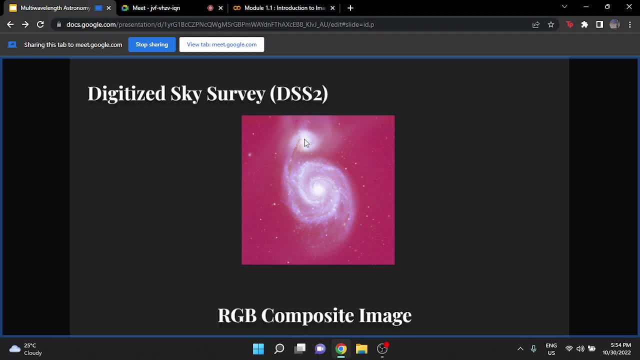 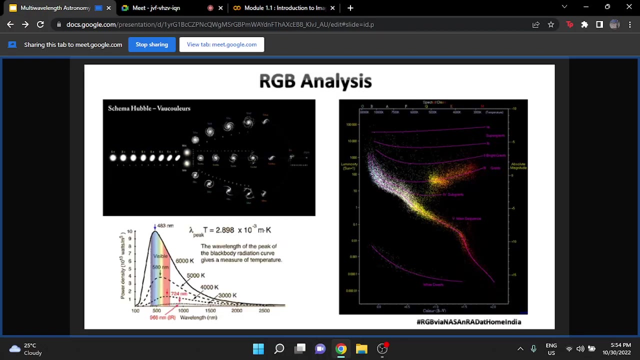 bigger spiral galaxy is eating up a small, like sort of a dwarf galaxy. So all of this information is simply by knowing what band, what color corresponds to what survey. So now, this is true for any galaxy and any survey. So the analysis that you can do with this, whatever we did. 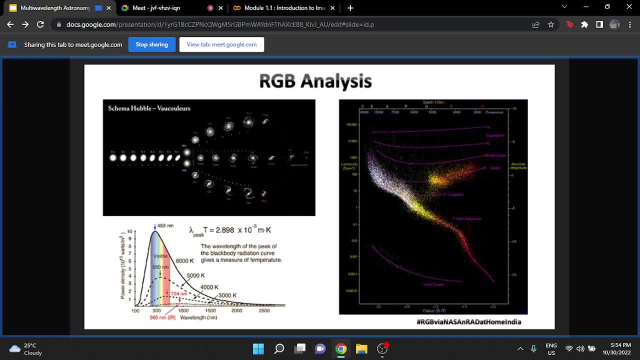 in the very first module is called as RGB analysis, And it is something very popularly done and very useful technique to do in extragalactic astrophysics. So by looking at the shape you can tell what sort of morphology the galaxy has, And there is actually a lot of star formation dependence on. 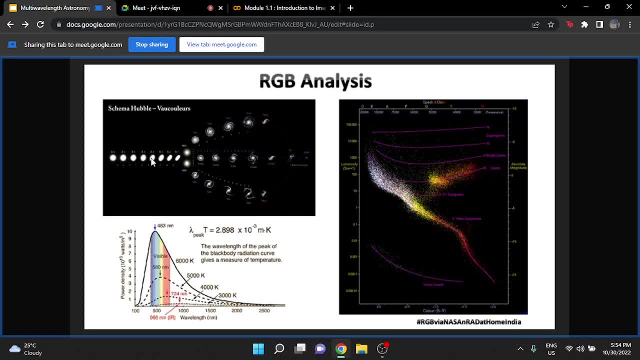 based on where you see the galaxies to be. So originally, what you see here on the top left side is the Hubble-Walker Tuning fork. it is actually the extension of Hubble's tuning fork. Originally it was thought that this has an 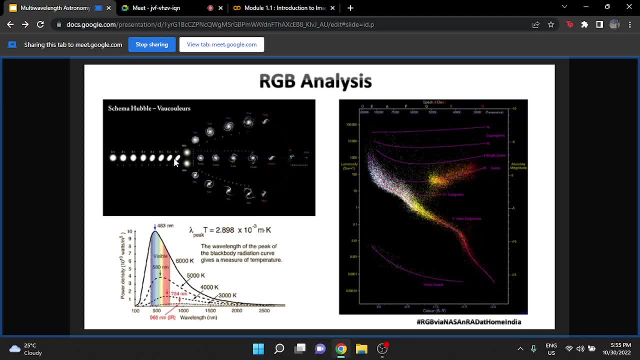 evolutionary phase, but later it was found that it's not doesn't correspond to any evolutionary trait, but it is a way to classify the shape of the galaxy. So it starts from very like circular elliptic galaxies, goes to lenticular galaxies all the way to spiral galaxies. So there's a 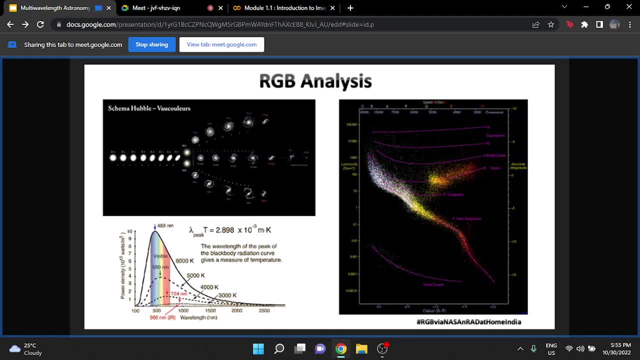 dependence on star formation And morphology also, which you could explore. You could explore if there is a presence of bar where the star formation is, And how do you look at star formation Using knowing which color corresponds to star formation. So now you know that blue corresponds to young stars, So wherever you see young stars. 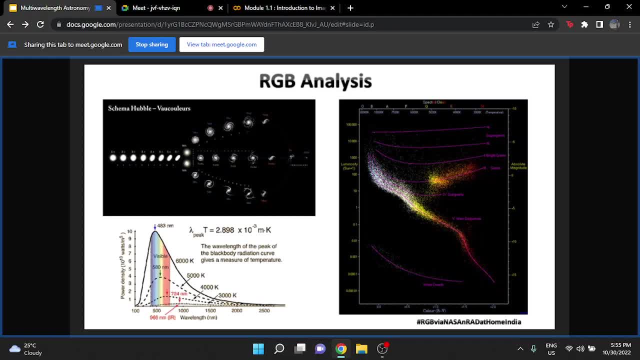 must be a star forming region. And all this is assuming that the radiation is from the radiation mechanism that is causing the radiation is blackbody, which is a good approximation at this level. Now, knowing where the galaxy or the stellar population that you're seeing falls in the H-R diagram, it's okay if you. 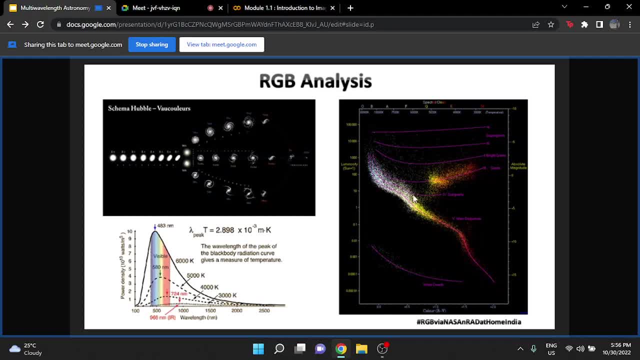 don't know what is H-R diagram. So this, what you see on the right side, is the Hartspell-Russell diagram or, shortly well, H-R diagram. It essentially gives you a relation between the galaxy's color and luminosity. 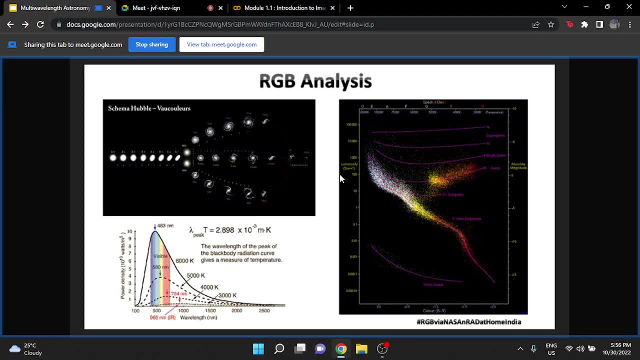 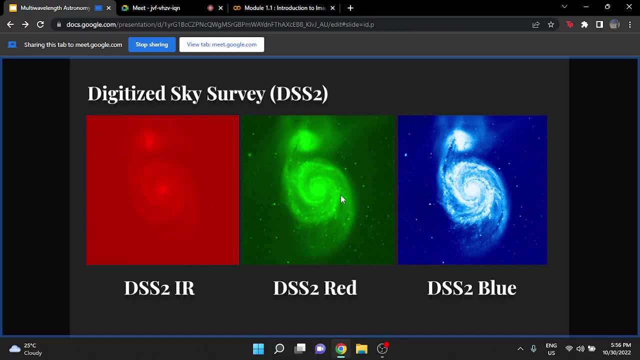 So a color of a galaxy is the difference in magnitude between two filters. For example, we used, you know, the DSS2 red and DSS2 blue, right? If we subtract these two, the magnitudes measured in these two filters, we'll get a quantity. 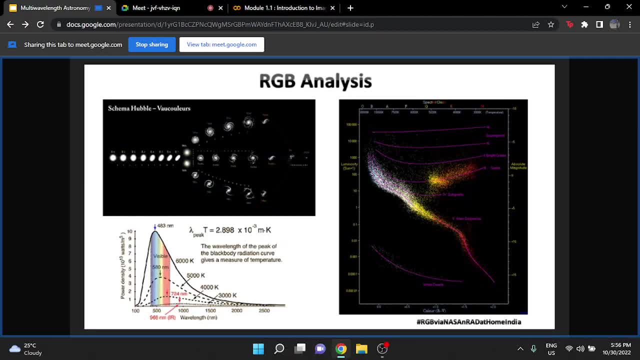 defined as color, So it is not has much to do with the color that we talk about, but it is essentially telling you whether it is bluer or redder, And that has a lot of significance. So if you understand H-R diagram, if you do a very basic look at the Hubble sequence, you can get the 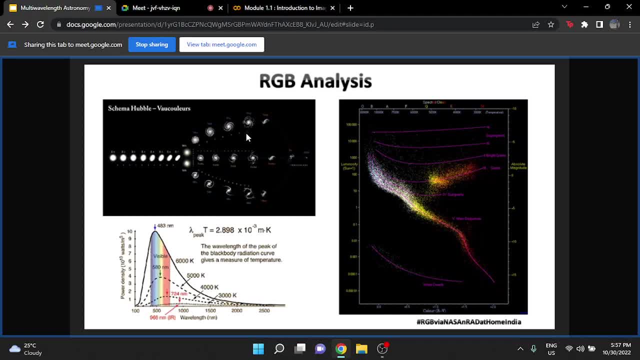 shape of the galaxy, which will tell you sort of which phase the galaxy is and what sort of star formation to expect, And from the H-R diagram you can find out what evolutionary stage the star stellar population that you're observing is in. So all this is simply by knowing what your image was. 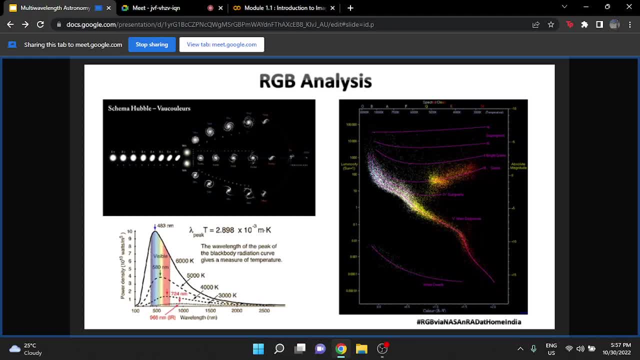 used to make and which is exactly what you did in the first week. Also, the puzzle is just to keep you interested in the workshop and to make our job of analysis. So all this is simply by knowing what your image was used to make and which is exactly what you did in the first week. Also, the puzzle is just to keep you interested in the 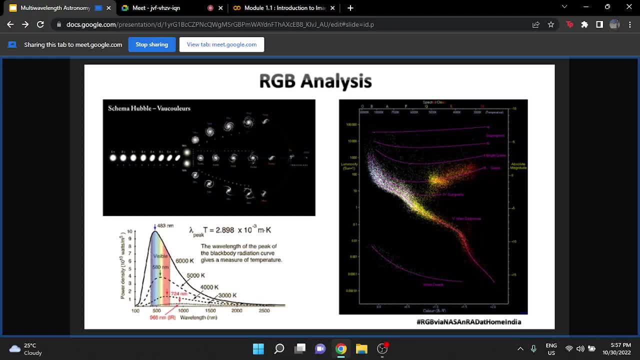 analysis, analyzing UZ, But the exercises are meant to just teach you how to acquire the data. It's sort of like teaching you giving your tool and telling you what to do, how to use the tool. but it's up to you how you use the tool, So you don't always need like a step by step explanation of what the code is doing, because I believe, like at the modern astronomy, you will be. 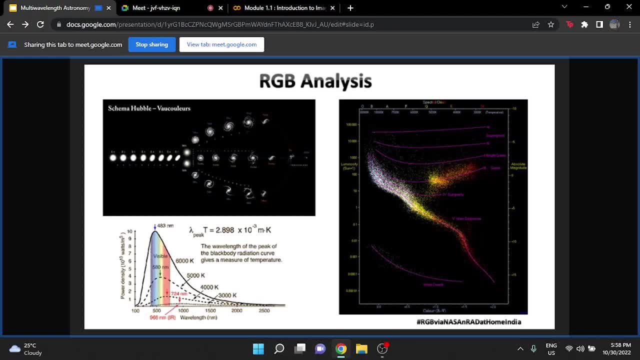 forced to use a lot of packages and most of the time you won't understand what is happening in the underlying code. For example one: what do you say? One function that you must have used in your module one is make looked on RGB. 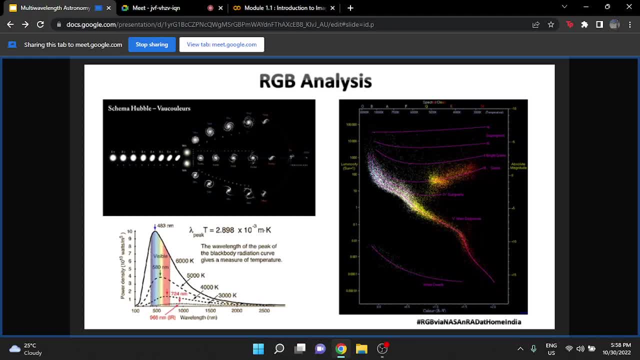 So there actually goes up quite a bit of data reduction, clipping processes, which goes behind the image. but you saw that we were able to reproduce a percentage of that using our normal RGB image making method. so you don't always need to understand how the code is working, but it is. 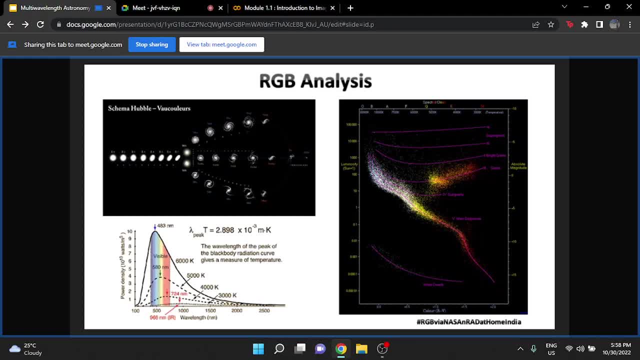 very important to learn how to use the code. so if you should be able to use a package, even if it is, if nobody is coming to you to teach you, this function does this. this function does this because that is not the logic of learning programming, that we are only learning the. 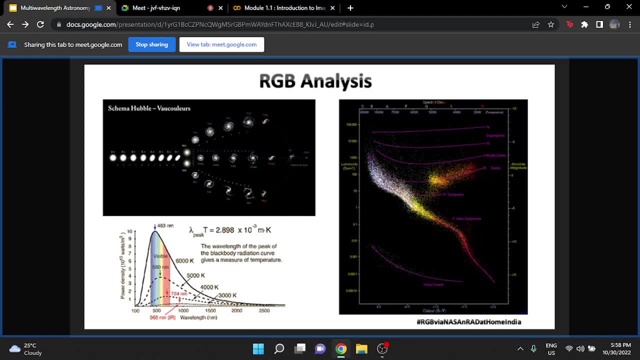 program, which is actually a very easy task to do because you can simply tell this function corresponds to this. this gives this result, but the amount of knowledge you get by using that package, in your own sense, making mistakes- you can't have that from simply like learning the. 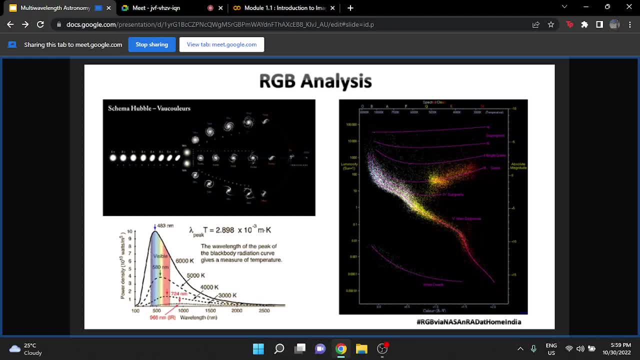 program. so, to conclude, the first module that you did essentially grasps and give grasp the elements that are required for rgb analysis. so what you can do is now that if you have complete at the module- which i'm happy most of you are, you can actually apply what you learned into any 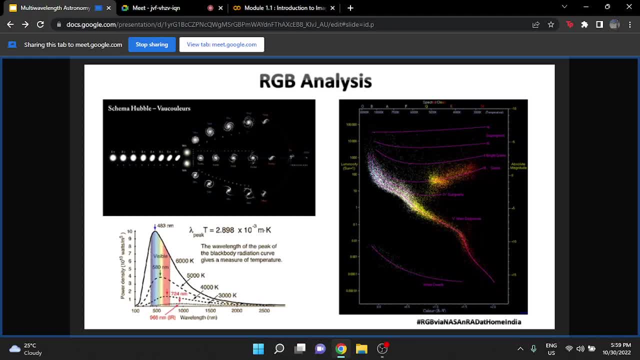 number of galaxy you want. so in this, in the module you only used, looked at couple of galaxies and sources, but you can make rgb images of, say, some five, six galaxies. look at its color, look at its shape and try to understand what it, what it means like. is it merging, is it interacting? 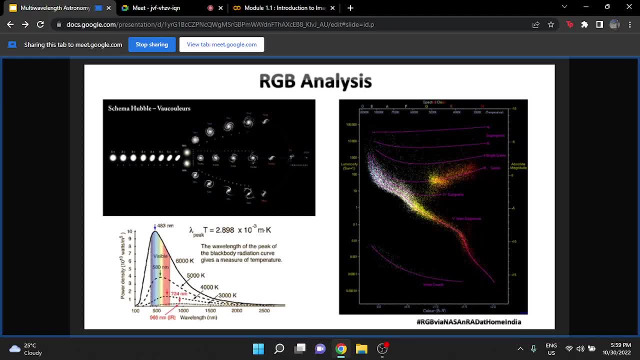 do you see star formation where it is not expected? now, to know where the star formation is, expected that you will have to do a lot of literature survey, because a lot of has happened in the last like century in the field of extra galactic astrophysics. but what? through this course and this first particular module you have 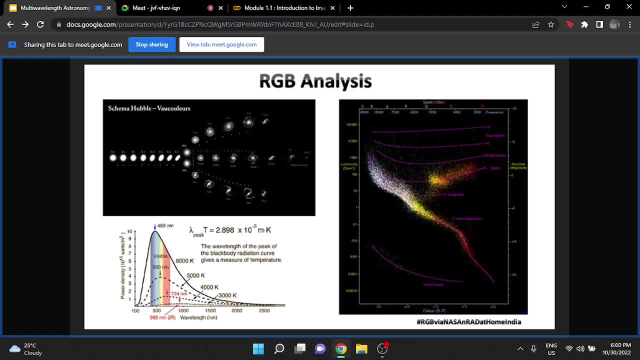 is a tool to make those images. now, irrespective of which project you are doing or which extra galactic science you are requiring, you can make these rgb images. for example, say you're studying star formation due to merging systems. you can use same rgb routine. you can use the uv filter in the 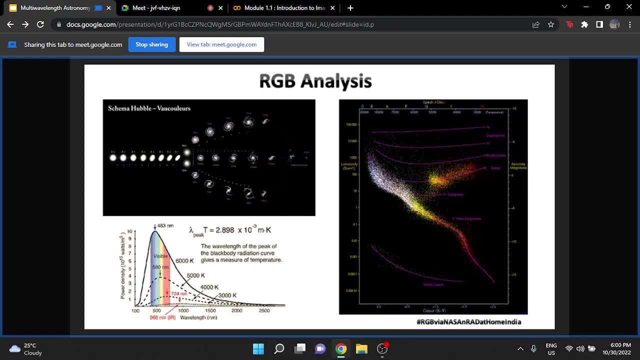 blue band and study star formation. similarly say you are looking for older stellar population you can look, at which all galaxies look very red, so it also could be because of dust and other properties. but essentially, now you have a method and a technique that will make you, that will help you. 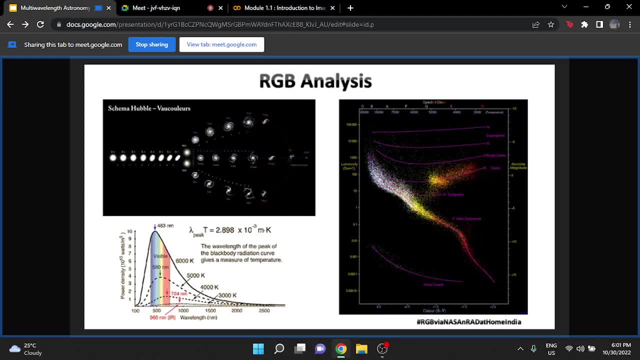 analyze an image in a more quantitative way. so now, whenever you look at an astronomy image, rather than admiring what the physical features of it, maybe you can look in the description which wavelength this corresponds to and what temperature is it and what information can you gather from it. so with that, i have met the goal of what i wanted to tell you with this. 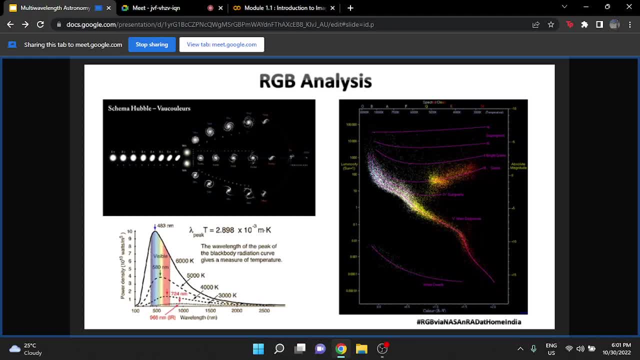 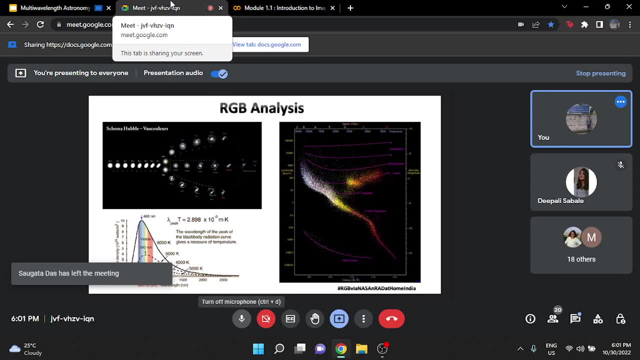 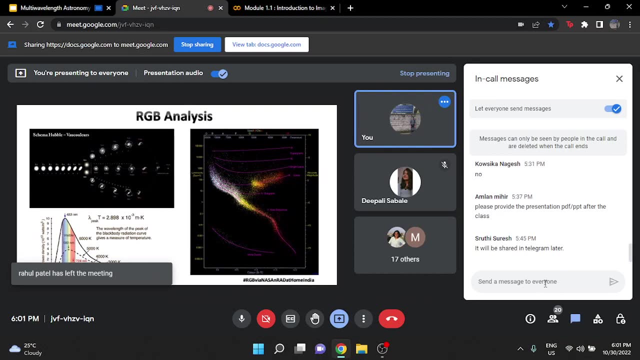 multi-wavelength astronomy lecture. so if you have any questions with anything that i've covered so far, you can ask me right now. or did everything just go over your head? so so spl20. so if yes, then you can draw a s Hess. do you think this is gonna help you say more questions? do you think about this? i don't think this is going to be a big deal. with anything that i've covered so far. you can ask me right now, ask me on the description, because i just think that almost everything i've covered at the end of the lecture. so did you all understand at least? like some say, 70 percent of the lecture will give you a possibility of questions. 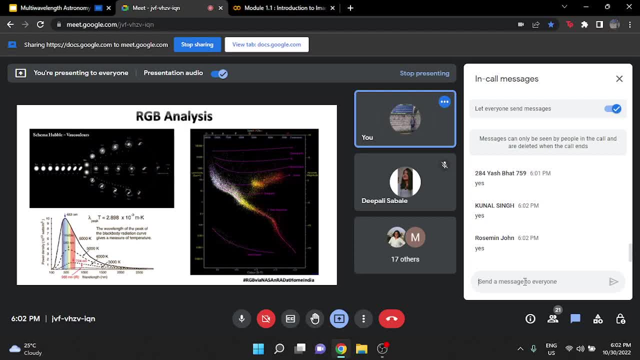 So do you think, if I give you a galaxy name, I give you a galaxy source, I gave you its data, you can make RGB image and do the analysis that I showed you right now? If yes, then you can drop an yes here again. 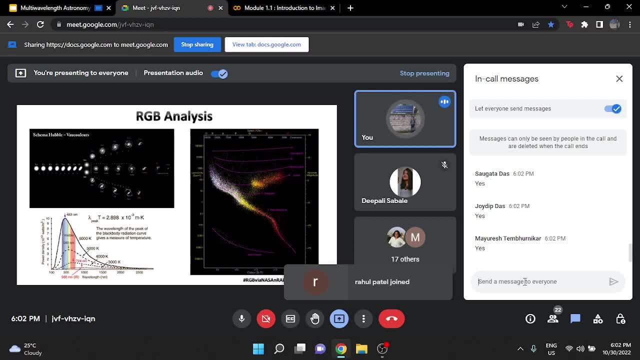 Like, if I give you a source and give the image, can you do RGB analysis? I have one. yes, for RGB. Yeah, probably. yes, we can do That's good. So does anybody want to discuss the actual code, if you want, Because from my colleagues, what I understand, that most of you have actually finished the code and some of you actually have done more than like did very fast. 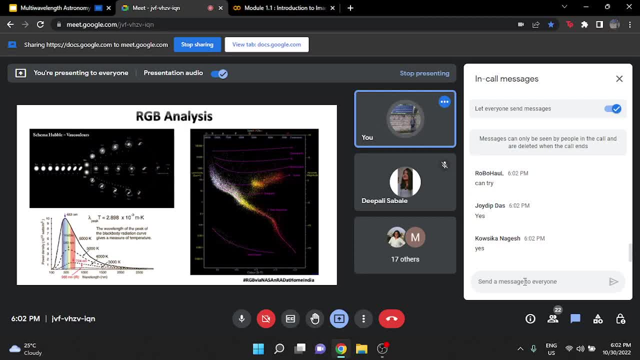 So I'd like to inform you that there is actually. if you can't do it, that's okay, But it's not like we won't give you incentive. It is for doing things faster. So the people who can handle the coding part well, we'll try to give them more theoretical aspects to work on towards the end of the course project. 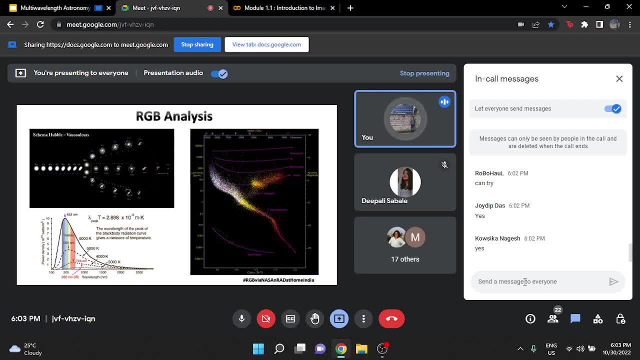 Because, like I said in the very first class, this time the workshop- we actually have a science goal in mind, So we'll be. we are hoping that at least out of your 23, a five of you could be a co-author with us in a paper. 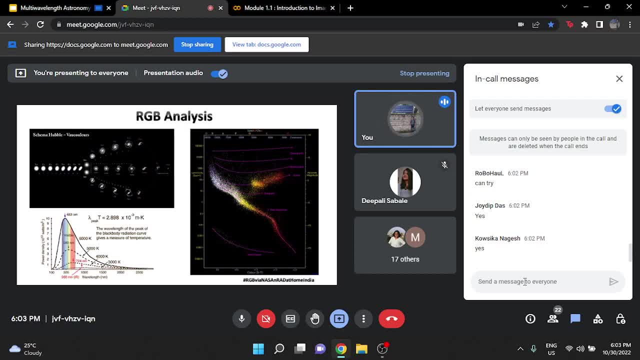 Because the project that we have in mind Has a lot of data reduction under uh it. it'll be helpful to get people who are good at this. So so the two good part advantages of this is, rather than just learning technique and applying it, you also get to apply it in a project and get it as a published result. 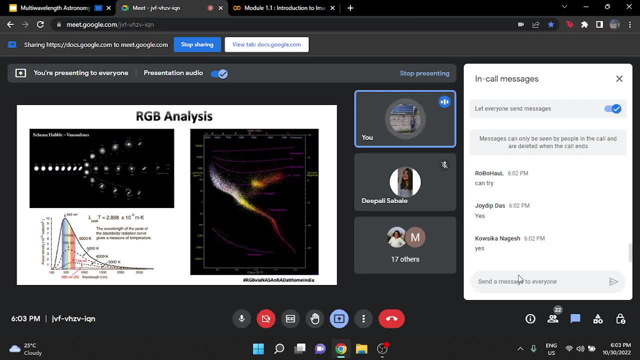 So if you are willing to put effort and do things faster and put more effort, you will be appreciated for that also, So you don't have to worry about that aspect. So Does anybody have any doubts about the RGB analysis, multi-wavelength astronomy or even coding doubts? you can even tell. if you are completely clueless about everything, you have not understood anything and haven't started yet. even that is fine, because it's still not late, because from the second week onwards we'll actually be targeting very specific topics, very specific packages that will lead to our final project. 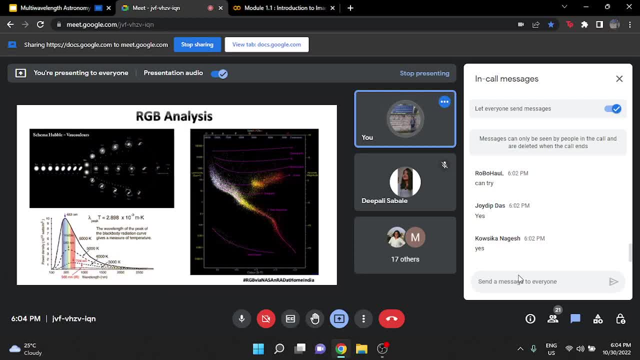 So if you have any doubts, you can clear before we conclude the second week. and even if, if you want at any point more information like this on RGB analysis, you want more information on, say, radio astronomy, or you want more information on a particular package, can always say that also. 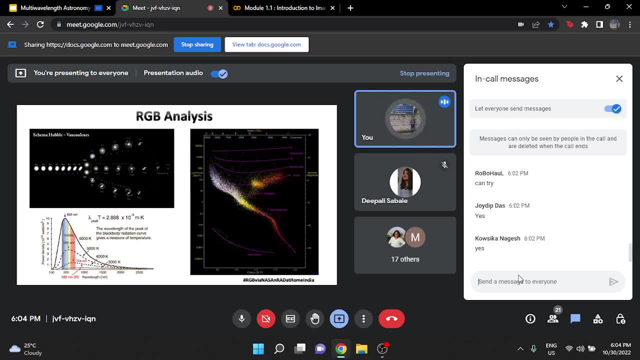 So any doubts? if you have no doubt, I can put a no in the chat. So I believe you understood everything. Yeah, Okay, In the previous assignment some of the codes that are actually given wasn't run properly. So, Deepali, can you like expand a bit more on that? 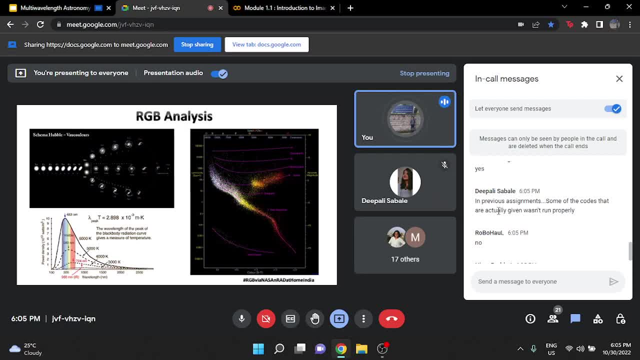 Maybe, like we can help you if it's a quick thing, maybe we can quickly help you right now. Or if it's a bit uh time taking, then one of us will like contact you and you can share the. So one thing I would like to tell you is the way, if you feel you don't have to feel shy to share if you don't understand anything, because the exact point is for you to try and make mistakes and learn. 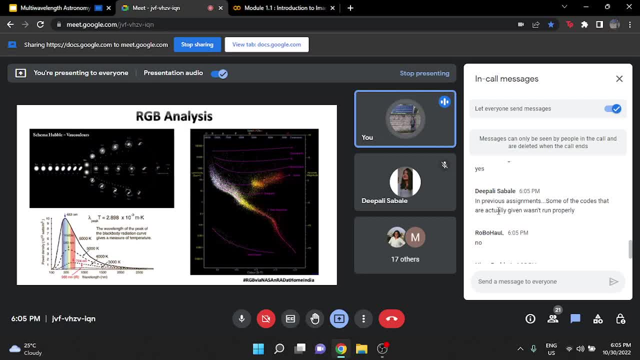 So please do try each module, each puzzle, because you, if you saw the first week module, you must be knowing it's not rocket science. whatever we show in the previous code is what we ask again repeatedly. So, Deepali, can you tell me, you can unmute and tell, or you can unmute. 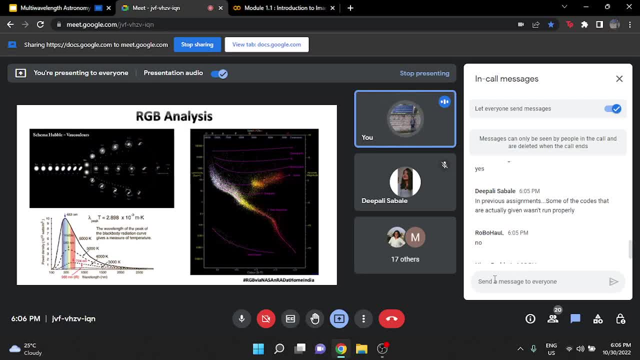 Okay, Okay, Okay, Okay, Okay, Okay. Take, type it in the chat box Also like which exact code: Hello, Okay, I'll present the collab notebook. So if you have doubt in any section, you can. So yeah. 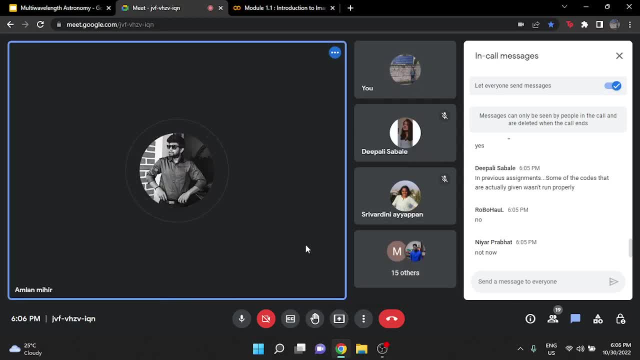 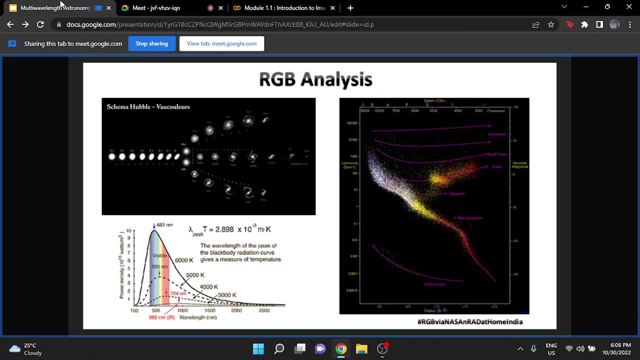 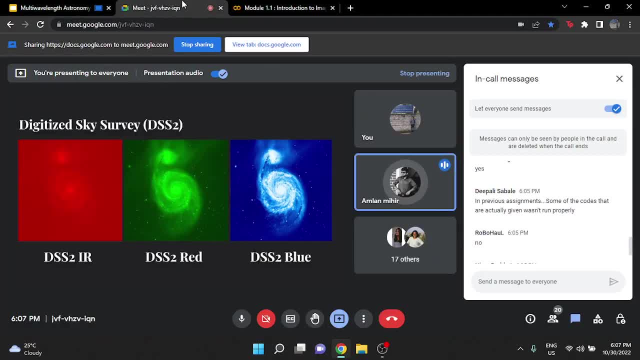 Yes, sir, It's, it's the right. yeah, The right, Yeah, Yeah. Can you have it on the left side? Yeah, Yeah, Yeah, Yeah. If we are looking at the IR image, see, IR is not visible to our eyes, so we should get totally- I mean nothing- data. it should be completely blank. 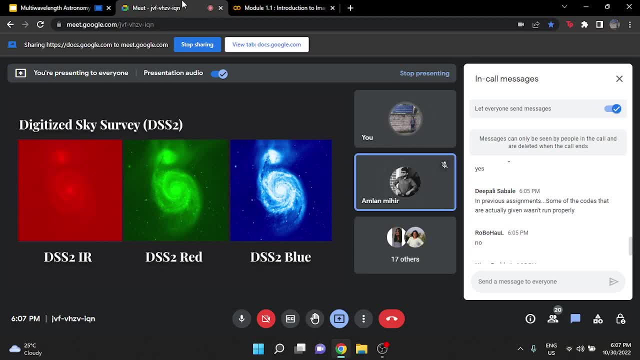 We are still able to see something. so how is that possible? Yes, so here we are not looking at the galaxy. we are using a telescope which has a detector. that detector can actually see IR. Now the detector is what is observing. what the detector gives us output is a 2D matrix with numbers. 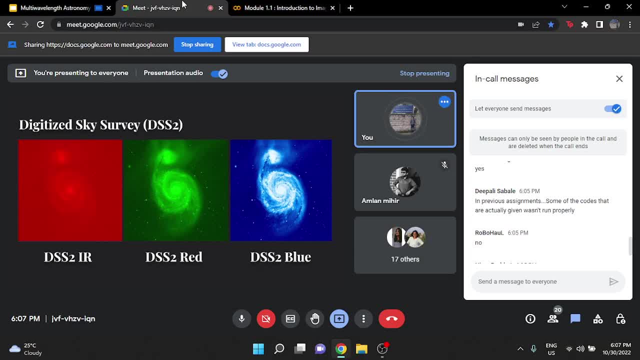 Now that does not have any information of colors, it is just a detector, just a 2D matrix with numbers. So the reason we are able to see IR is because the detector can see IR. So the exact same thing works with all observations. we cannot see radio, but we can make detectors which can see radio, same with X-ray or UV. 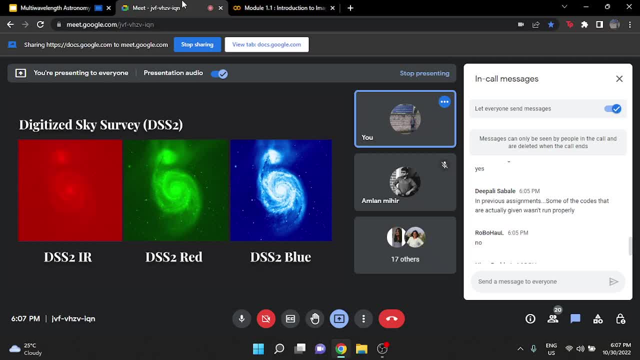 So does that clear your doubt? Amlan, Yes, Great, Yes, that is. even 60% is good. any person greater than 0 is good. So you have so. the reason it spans one month is: see all of these lectures and coursework. these assignments can be done. 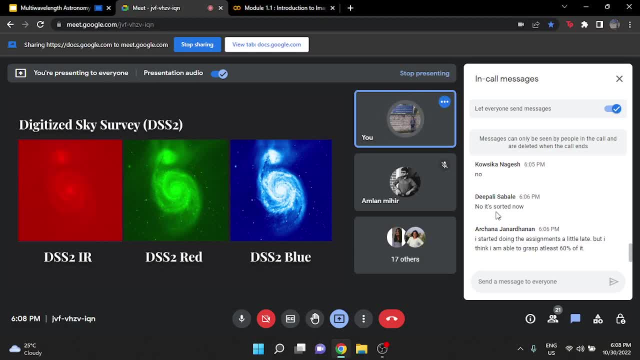 In a span of, say, 5-6 days. But the entire objective is to so that you actually benefit from doing these exercises, so that we are available to you 24-7 to help you with the science and the coding part. So any sort of progress is better than no progress. 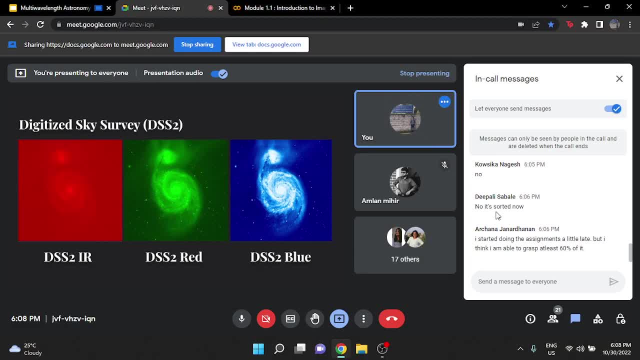 So you do not have to worry about your pace if you are a bit slow, that is okay. So yeah, Sir, you said that based on our responses or In this assignments, there would be Assign some last week project. can you clarify on that? 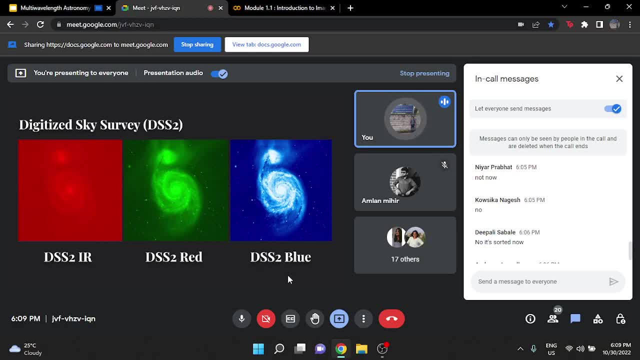 Yeah, sure. So what we every year do is we divide you into groups And each group will be assigned a specific topic, and we divide the group based on such that we shouldn't- we don't- want everybody in the group to be really good. 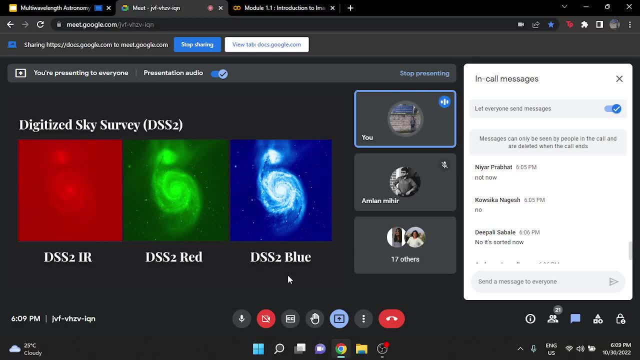 That that means it will give a selection bias to the other groups. So what we do is based on your performance. We'll divide you into groups such that all groups have equal performative capacity and the topics are also chosen based on like how well you performed in the group. 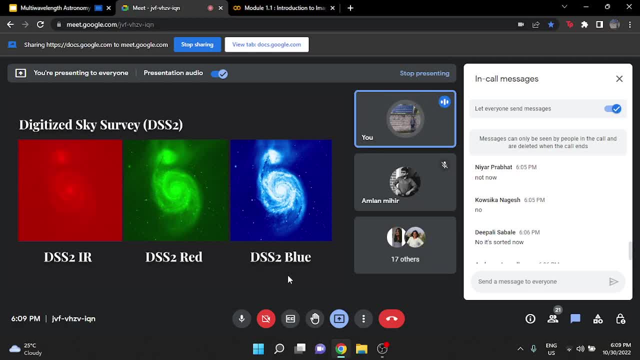 So we don't want you to give you a project which is too difficult for you because it's like some people would be coming from a very good programming background, So we can't give them a very highly physics oriented project. similarly, somebody coming from a very pure science background, we can't burden them with a machine learning or a deep 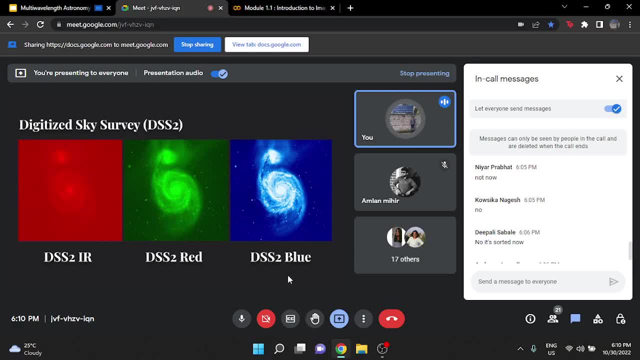 learning project. So the segregation is to your benefit. it's not like a person who does it first is better or a person who doesn't code well is bad. it's just that your feedback is very important for us to segregate you into groups. 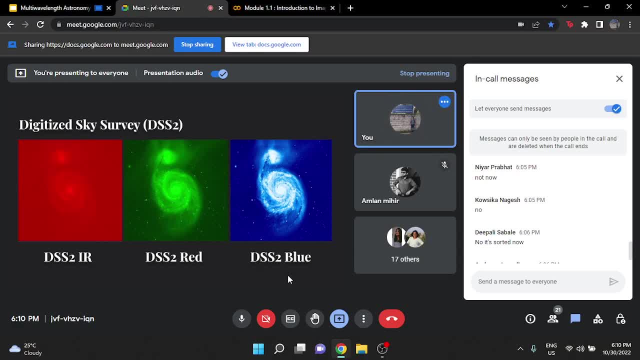 And this time the project, since it has a proper scientific goal. we are trying to make sure that the people in each group, the groups, do perform in a way that we can quantify your performance. So some groups will act as validation groups and some will be doing the training and some 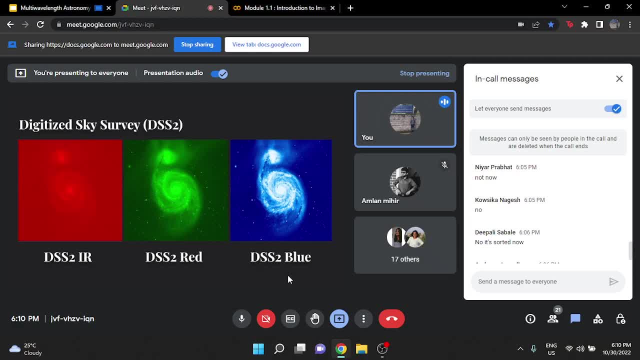 will be doing the testing parts. So, based on your coding performance and how regular you are, we just segregate you into groups. So that's essentially this. We just stuff it. I hope that was clear. Amlan, was that clear. 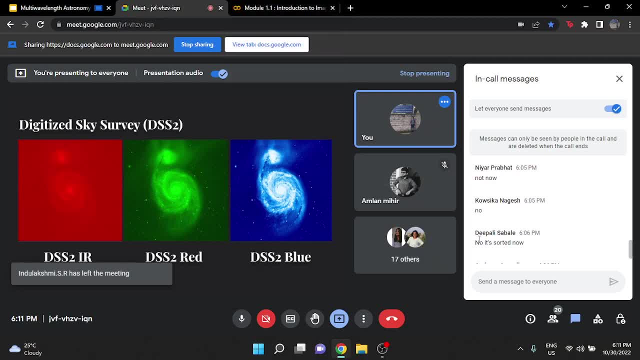 Yes, sir. So if you don't want to discuss the module right now, then you can drop a note, because I see it's been over an hour and statistics say that people can't listen to lectures more than 45 minutes. So I don't think like even if I go ahead, it will be of much use. 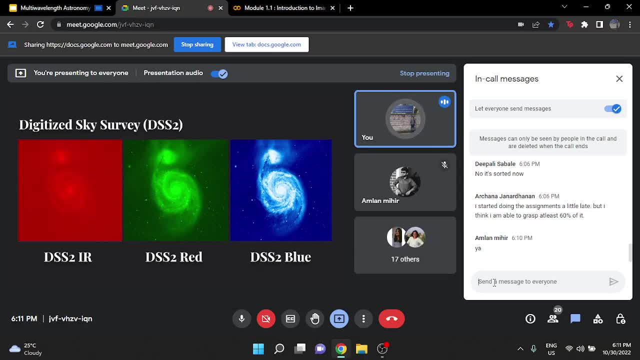 So do you want me to continue or shall we break for today? Drop a yes if you want a break for today. So I see two yeses. So that's it for today, Thank you, Bye, Bye, Bye, Bye, Bye. 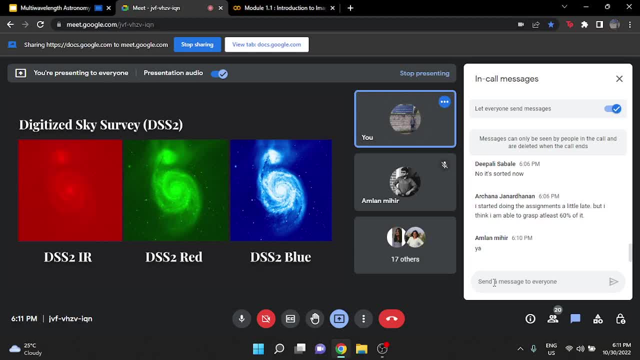 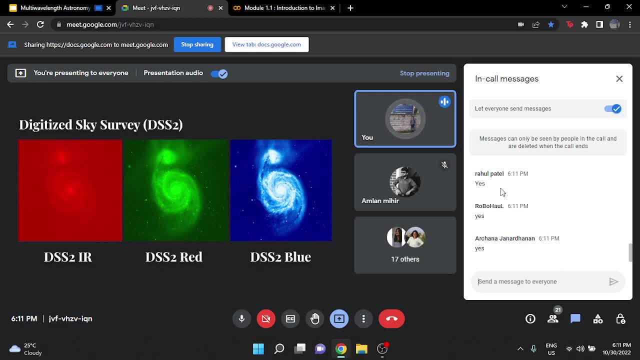 Are you ready for mandatory remove concepts from martial law? Yes, Okay, Tell you the rest of you want to discuss the module. If you don't want to discuss the module, then you can. Should we do? The thing is, let's do one thing. 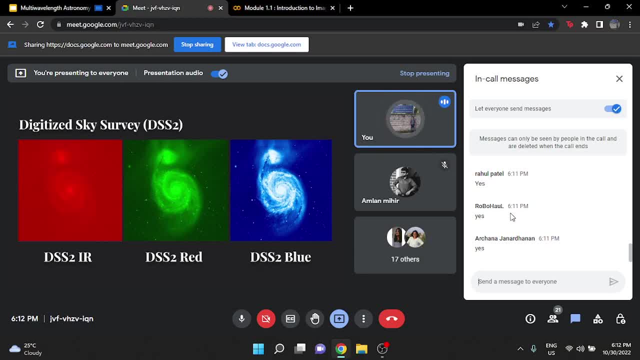 Let's break for today, because I think I assume many people will be submitting tonight And if there are people who still have problem with week one puzzles, we'll have them eating like this, specifically for tomorrow, because I think it's enough And it's not.